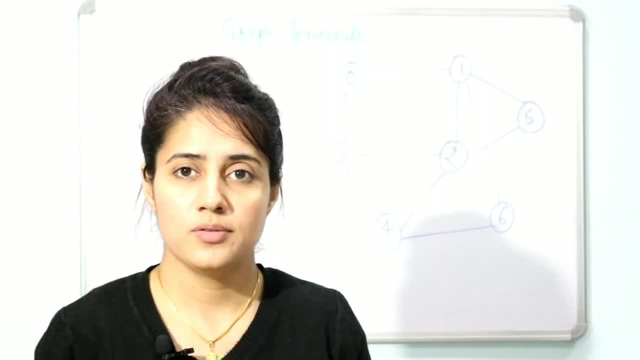 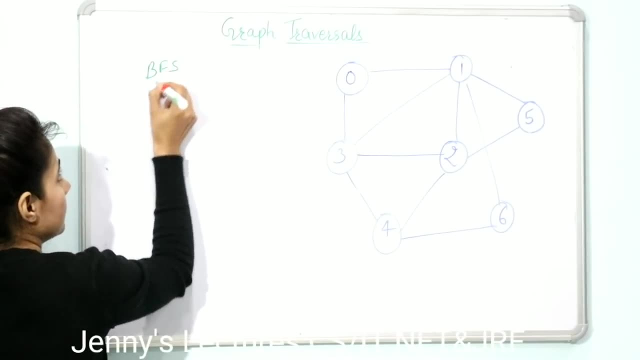 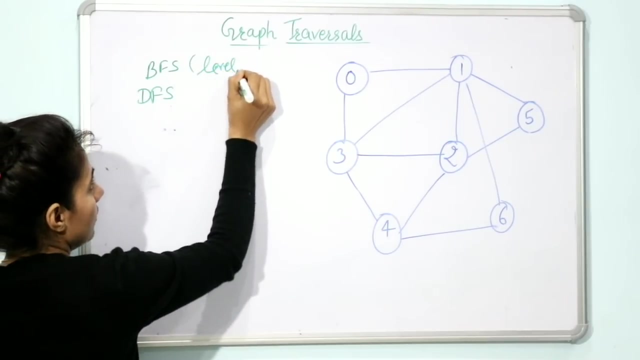 Hi guys, in this video I am going to discuss with you graph traversal techniques. Two types of graph traversal techniques are there: BFS and DFS. BFS means breadth first search, or sometimes it is also known as level order traversal, And DFS is depth first search. 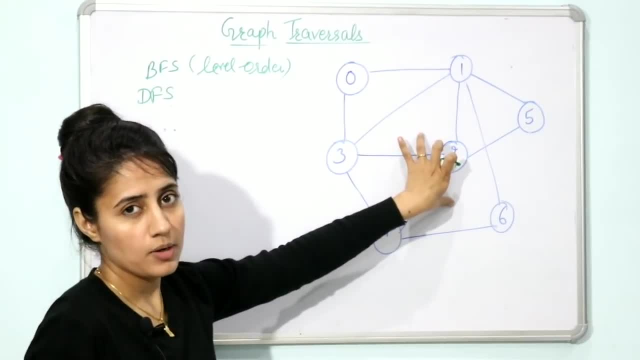 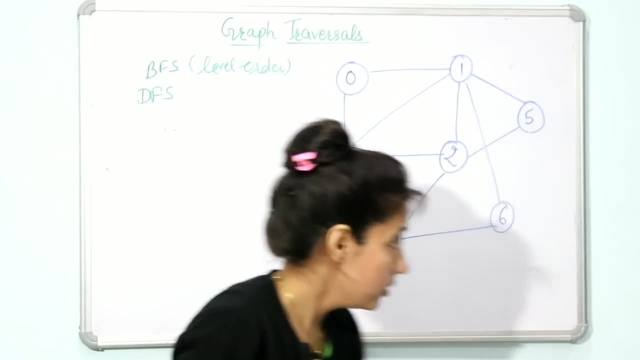 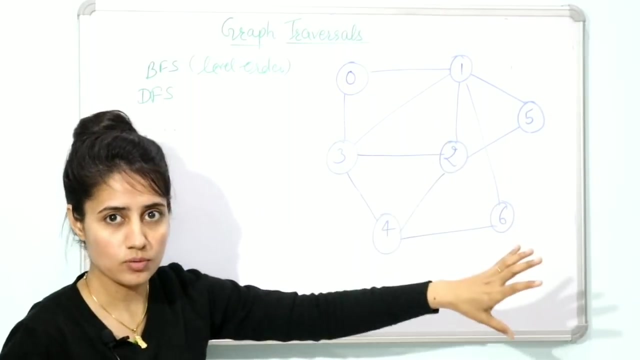 Fine, so we will take this example and with the help of this example, I am going to discuss with you the BFS traversal. Fine, in BFS traversal, when you will start, then you can take any node as a root node. You can start traversing this graph from any node. 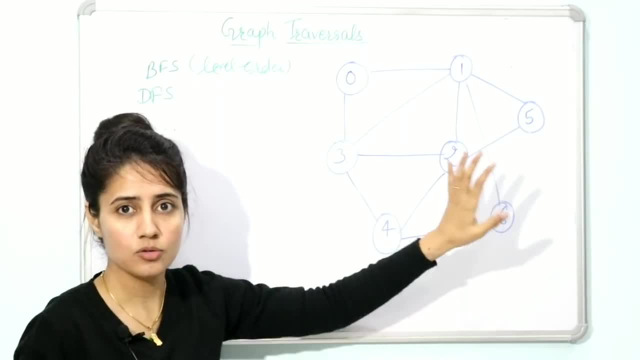 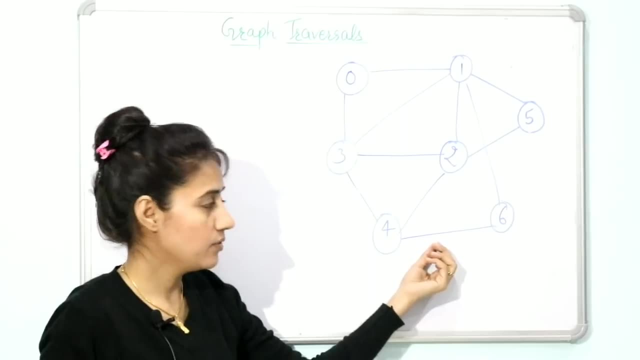 Suppose you can take 0, you can take 1, you can take 6 as a root node and you can start your traversal. Fine, but sometimes in question, if it is given that BFS traversal find out of this graph and considering 2 as a root node. 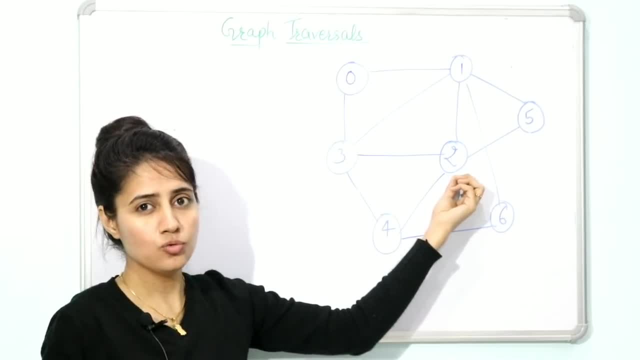 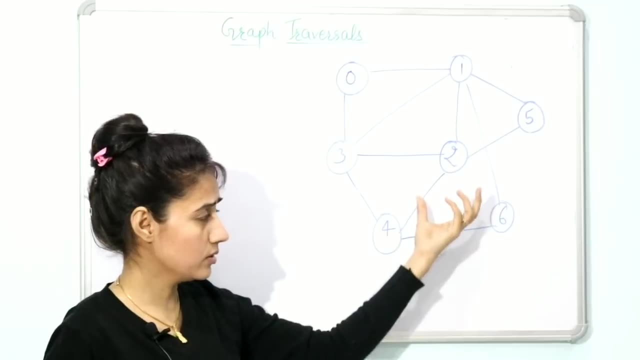 Then what you have to do is you are supposed to start From this 2, you will consider 2 as a root node and you will start traversing this graph from this node only Generally. suppose in this example nothing is given, then we will consider 0 as a root node. 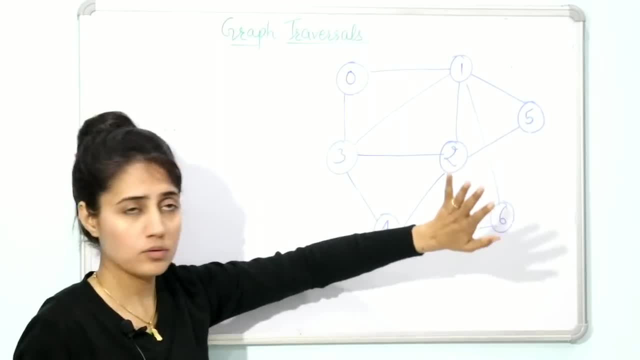 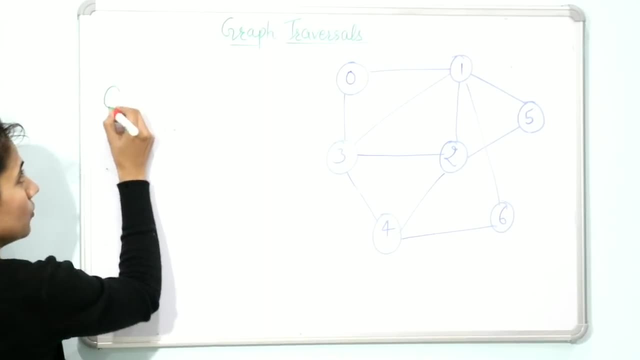 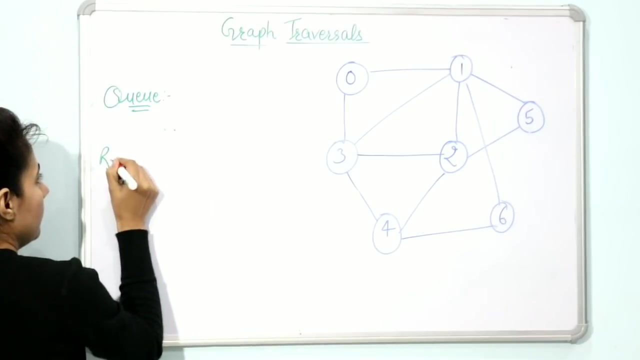 I am just considering 0 as a root node. You can consider 1,, 5 for any node. Okay, so for BFS traversal, what a data structure is used? that is Q. Q data structure would be used. Fine, And here you will write, will print the result. and this is our data structure, that is Q. 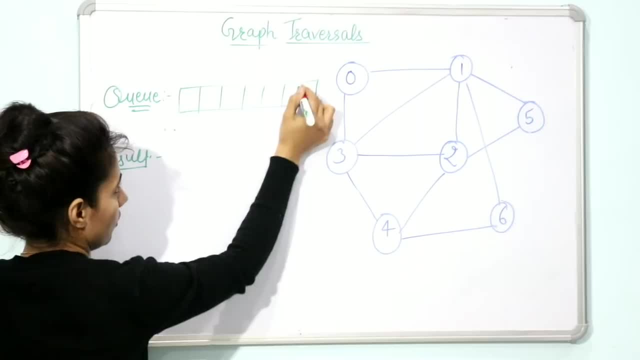 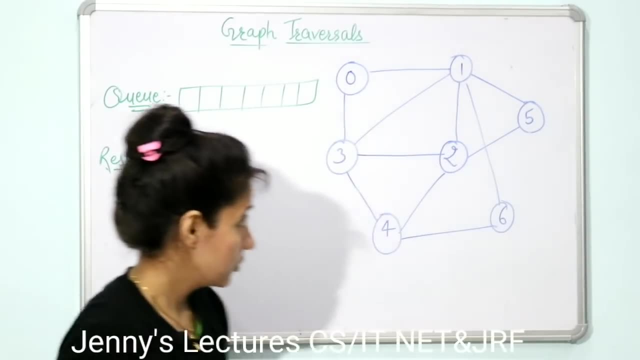 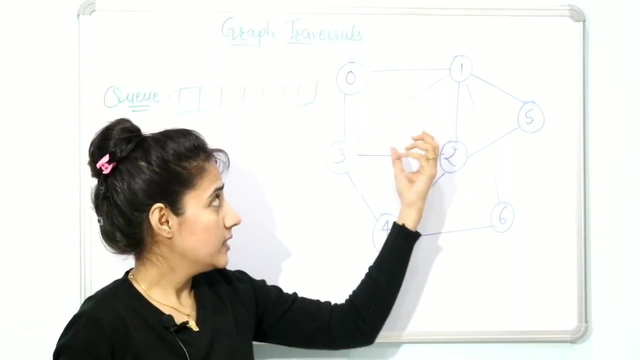 I hope everybody knows Q work in what fashion that is FIFO: first in, first out. Okay, so in this traversal suppose we have taken 0 as a root node. Okay, all the adjacent vertices of this 0 will be traversed first. Try to traverse all. 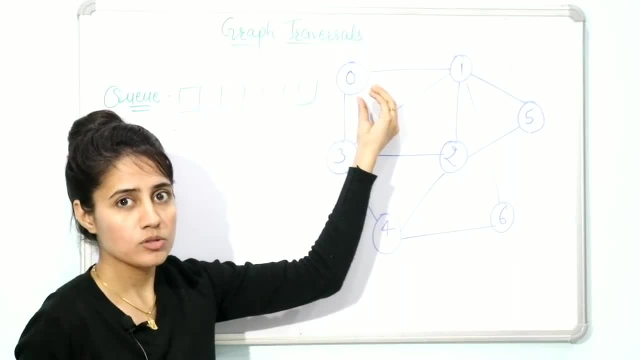 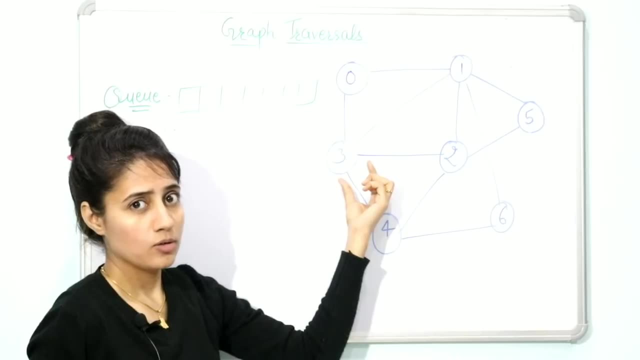 All the vertices as close as possible to the root vertex. See its close or its adjacent vertices are 1 and 3.. So 0 will be visited, after that 1 or 3, or either 3 or 1 in any fashion. 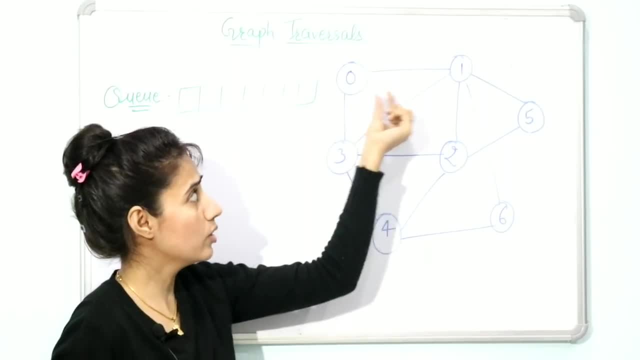 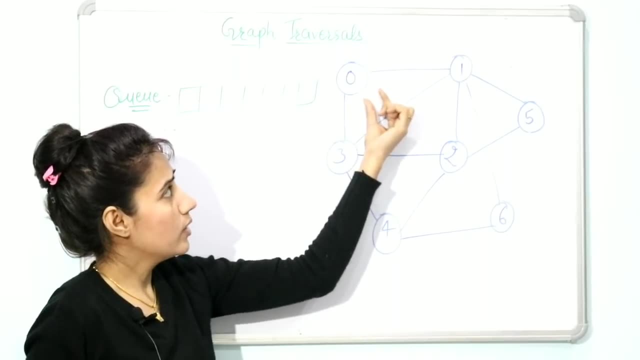 These will be visited. after that, you would move forward. It will not happen that after 0,, 1 is visited and then you would visit 5.. Okay, first of all, all the vertices will be as close as possible to this 0.. 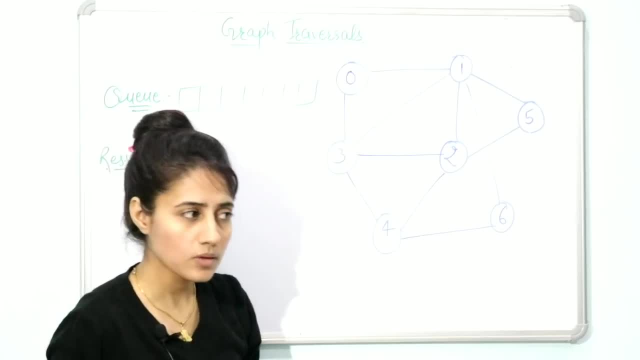 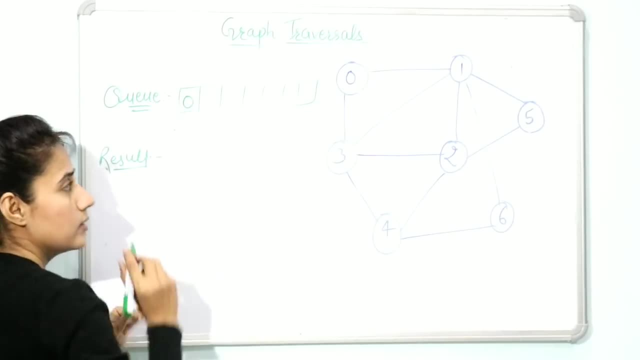 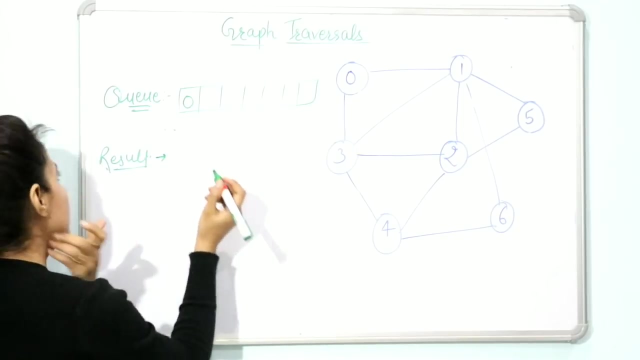 Those vertices. What is this? would be visited. Fine, Okay, Now, see, suppose we have taken 0 as a root node, So 0 would be inserted in this Q. Fine, Okay, Now in the result we have, suppose we have deleted this 0 and we have printed this 0 in the result. 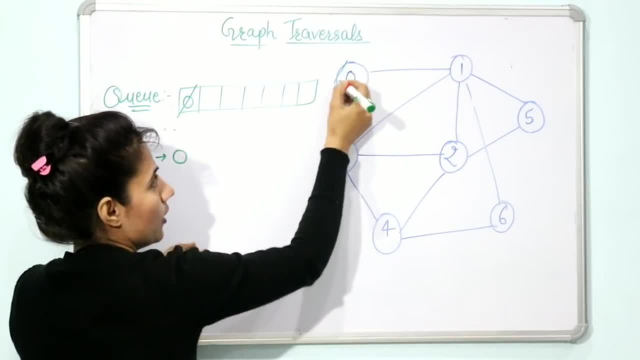 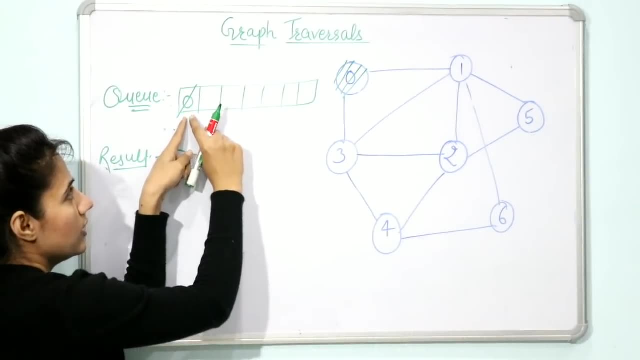 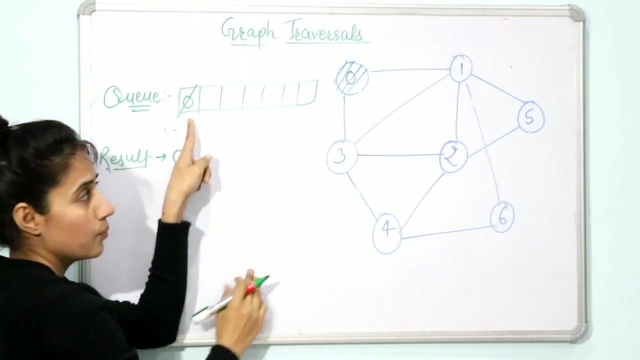 Fine. Now, as soon as the 0 is printed means 0 has been visited. Now, next thing what you have to do is, as soon as the 0 is deleted from here, all the adjacent vertices of 0 that would be inserted in this Q. 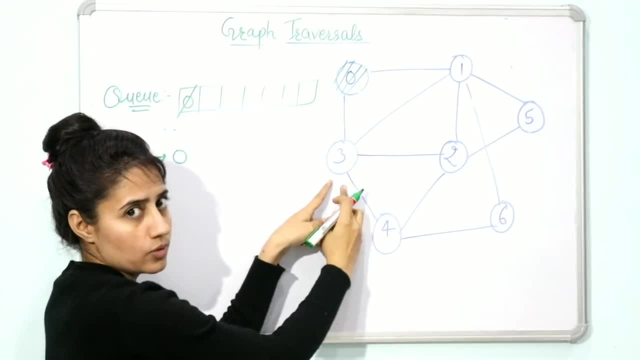 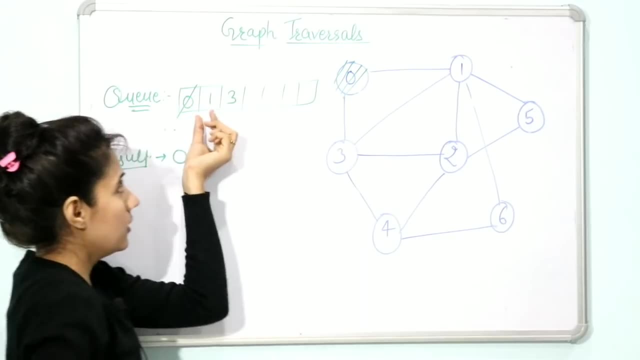 Now adjacent vertices of the 0 is 1 and 3.. Fine, Now 1 and 3 would be inserted in this Q, 1 or 3. It's not like 1 would be inserted and after that 3. you can insert 3 or 1, in any order you can insert. 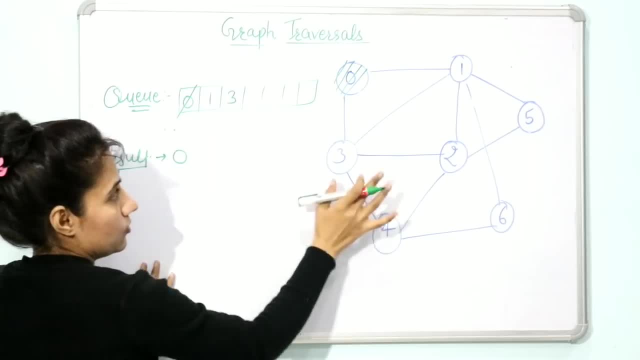 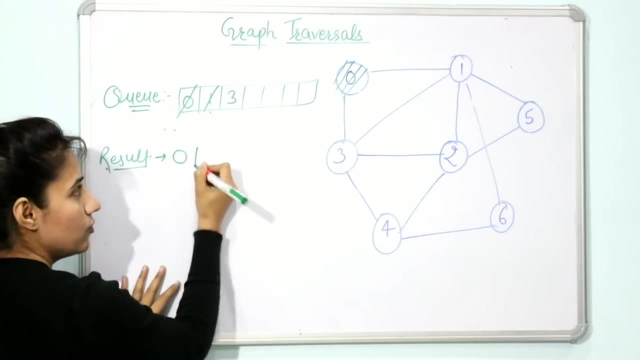 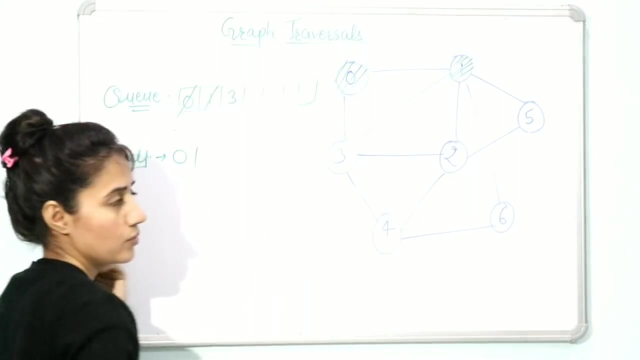 Fine, Okay Now. 1.. 1 and 3.. Okay Now. next is next element in Q is 1.. Now 1 would be deleted, and what 1 would be printed? means we have deleted 1, that 1 has already been visited. 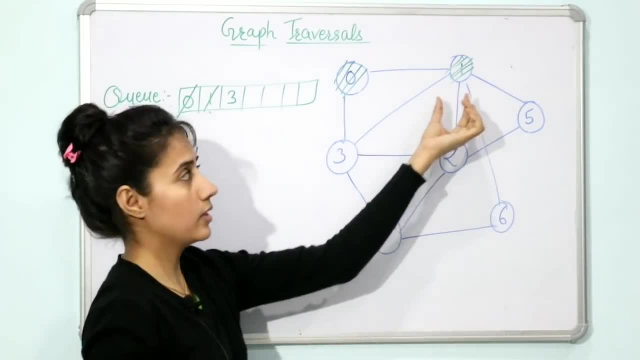 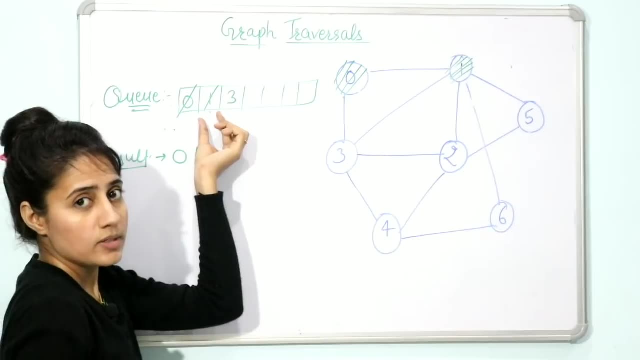 The same thing has been printed means 1 has already been visited. Now, next thing: what you have to do is all the adjacent vertices of 1.. All the adjacent vertices of 1.. Adjacent vertices Plus Unvisited vertices. Fine, 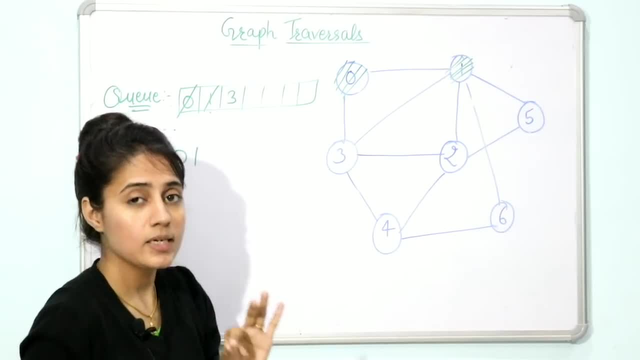 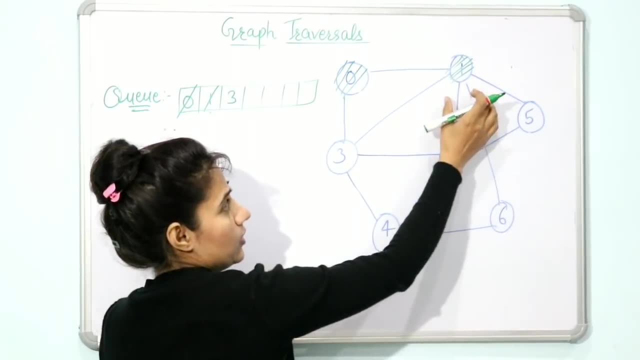 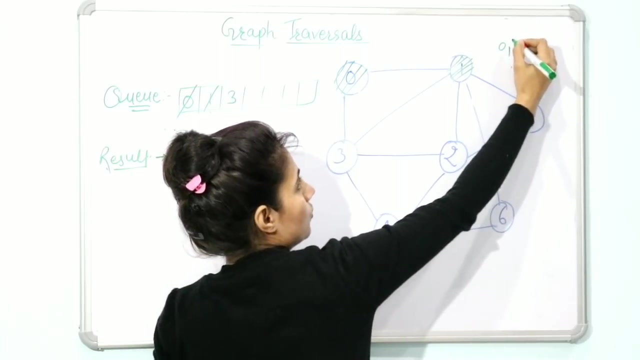 Adjacent unvisited vertices of 1 would be inserted in this Q. See how many adjacent vertices of 1 are there: 0,, 3,, 2,, 5 and 6.. I will write 0,, 3,, 2,, 5 and 6.. 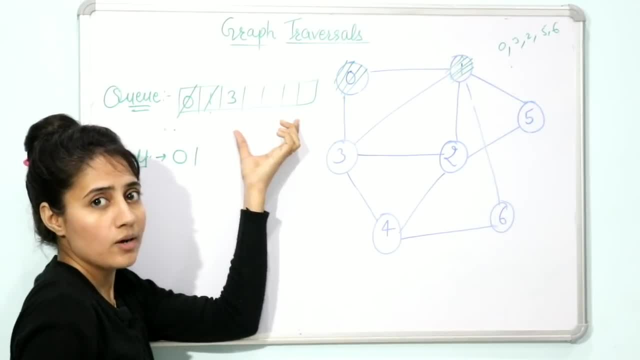 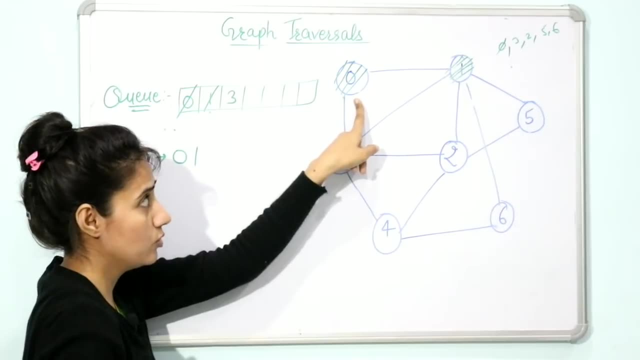 But what you have to insert in this? Only the unvisited vertices. 0 has already been visited. Fine, 0 has already been visited, So you will not insert 0 in this And 3.. 3 has already been inserted. 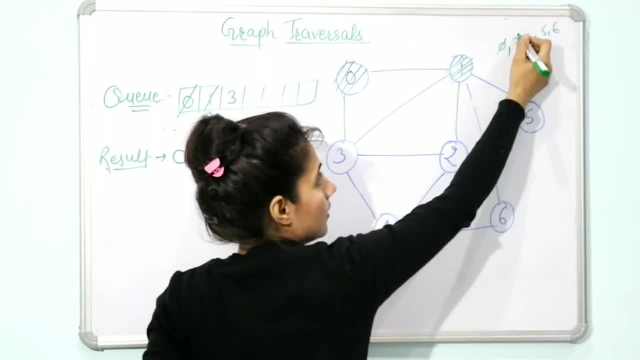 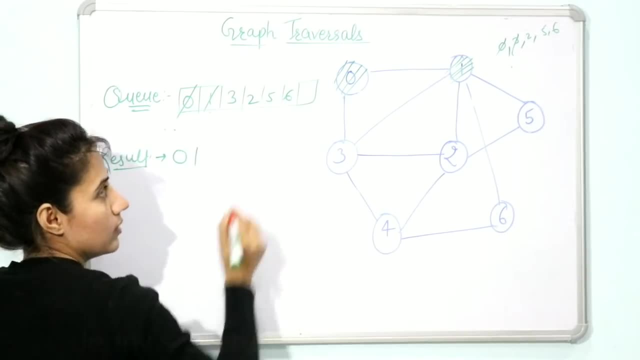 Fine, So you also do not have to insert this in this, Which will be inserted in this. 2, 5 and 6.. 2, 5 and 6.. You can insert 2, 5, 6 in any order. 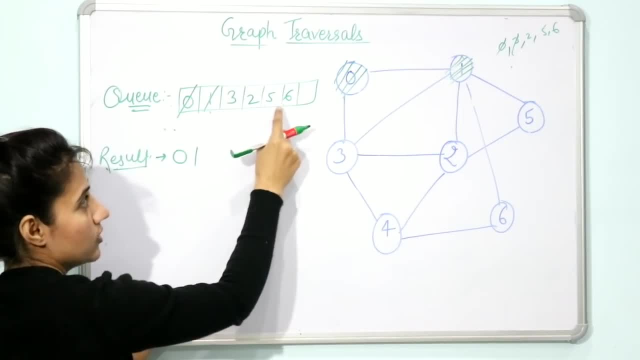 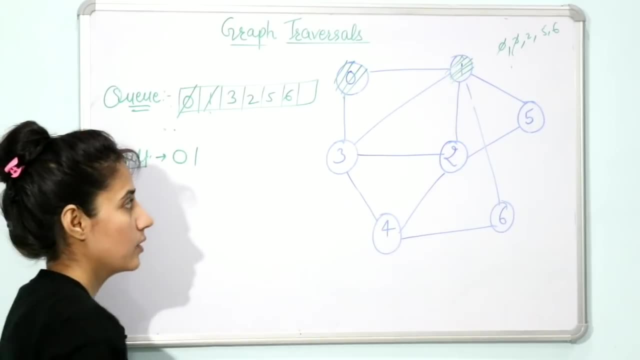 That is, You can insert 5,, 2 and 6.. You can insert 2,, 6, 5.. You can insert 6,, 5 and 2.. It is not compulsory that you will insert 2,, 5 and 6 only. 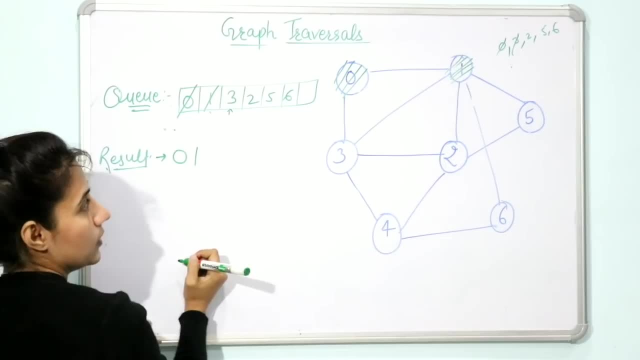 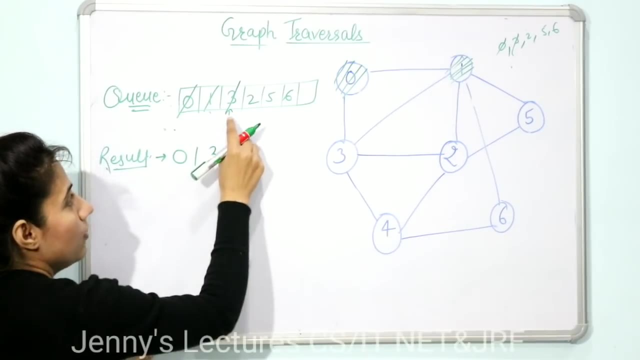 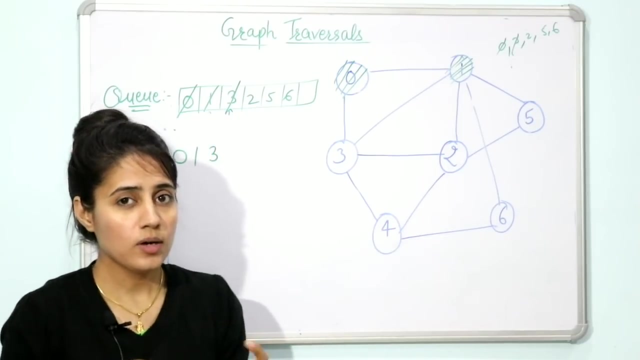 Okay, Now next is 3.. Fine, We have deleted 3 from here And 3 would be printed. And what are the adjacent vertices of this 3?? Find out those. See This, What we are finding out. 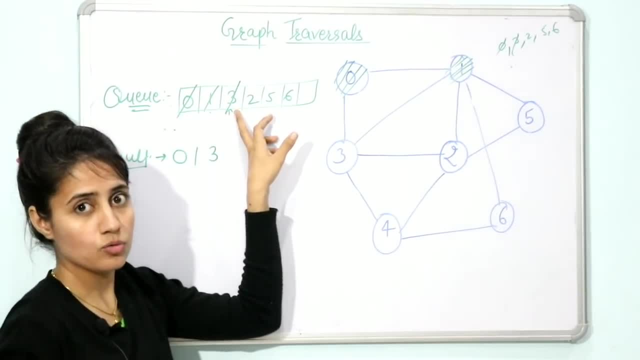 All the adjacent vertices of Any node. It is called exploration of that node. You are going to explore that node, Fine, Now find out the adjacent vertices of this 3.. Adjacent vertices of this 3 are: See We have printed 3.. 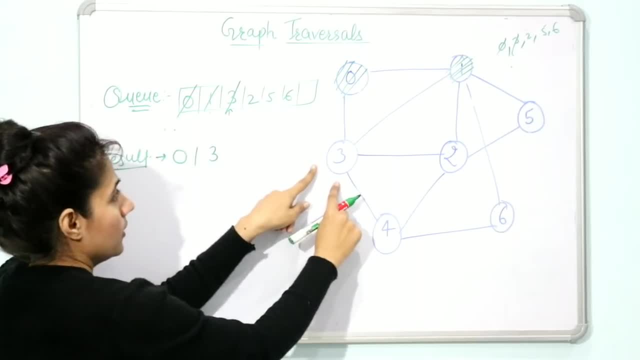 Means that has already been printed, Or you can say That has already been visited. This will be fine: 3.. What are the adjacent vertices of 3?? See, There is 0.. You have 1.. You have 4.. 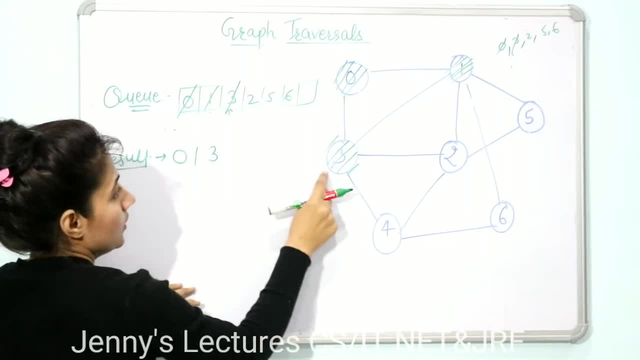 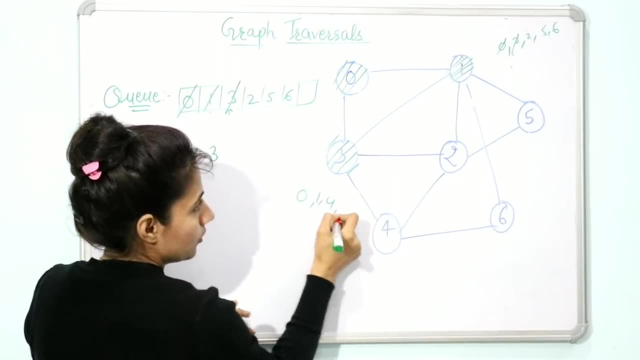 You have 2.. You have 3., You have 4., You have 5., You have 6., You have 7.. You have 8.. You have 9.. You have 10.. You have 11.. You have 12.. 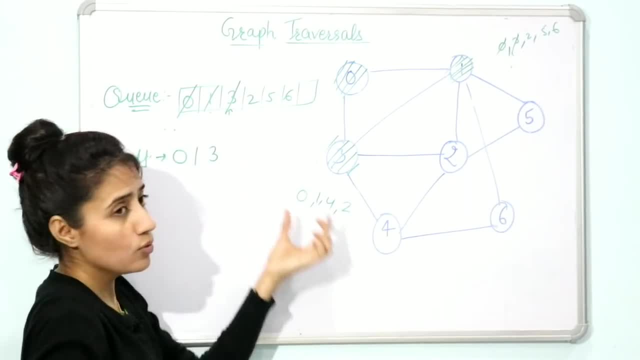 You have 11.. You have 11.. That in number 4.. Adjacent vertices are there, But which one you have to insert? That has not been visited, See: 0 has already been visited. 1 has already been visited. 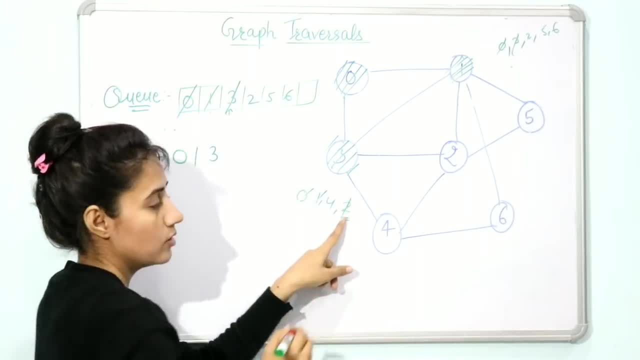 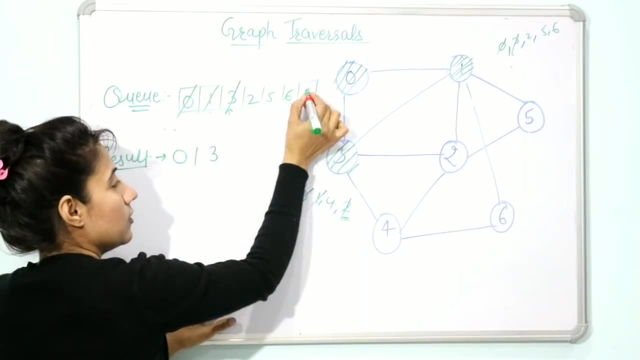 And 2 is already there in this queue. You would not insert 2 again. you don't have to repeat. The only element left is that is 4.. Now, 4 would be inserted in this queue. Fine, Now check next element. 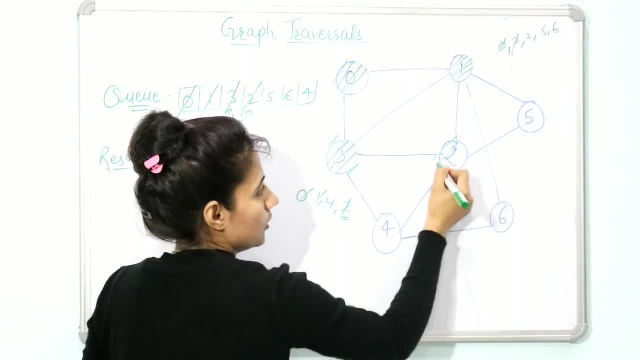 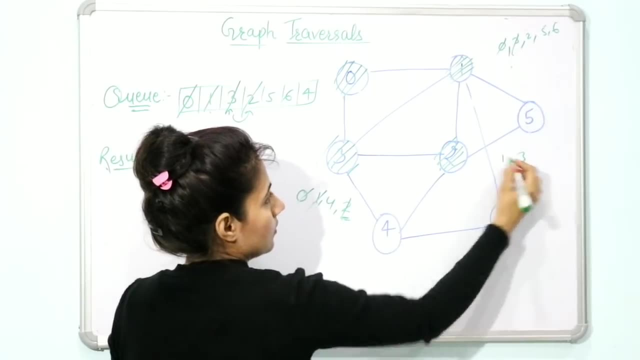 That is 2.. 2 would be deleted. be printed means 2 has already been visited. now find out: at the same element of this 2, at the same element of this 2 are 1, this 3, this 4 and this 5: 4. 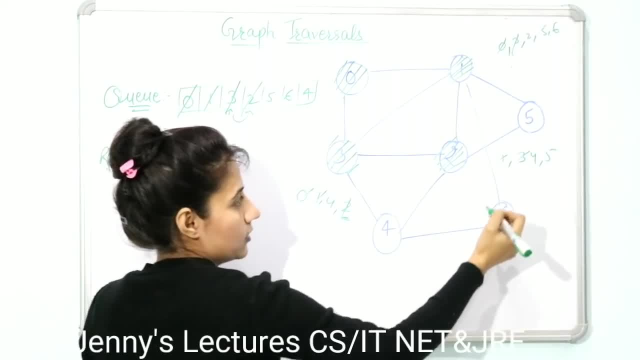 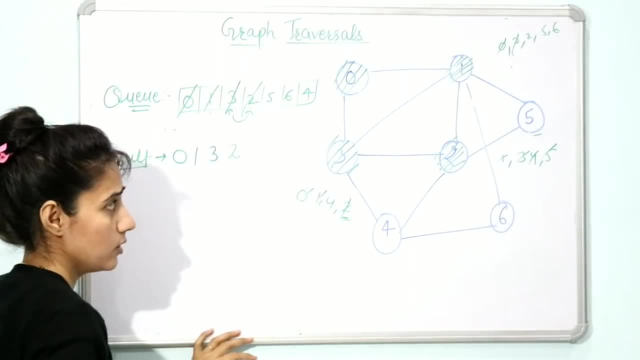 element we have. 1 is already visited, 3 is already visited, 4 is already there in this queue. only left is 5. no, sorry, 5 is already there in this queue, so there is nothing to insert in this queue. okay, now move to the next part, the next element. 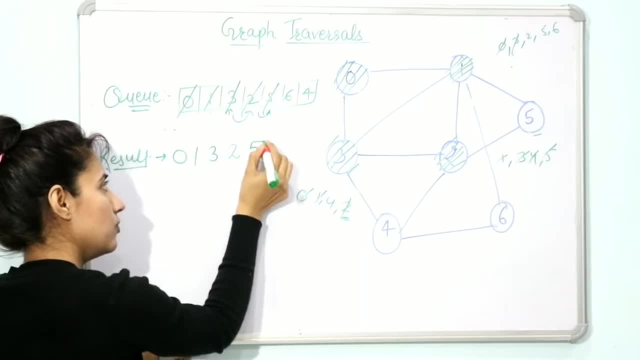 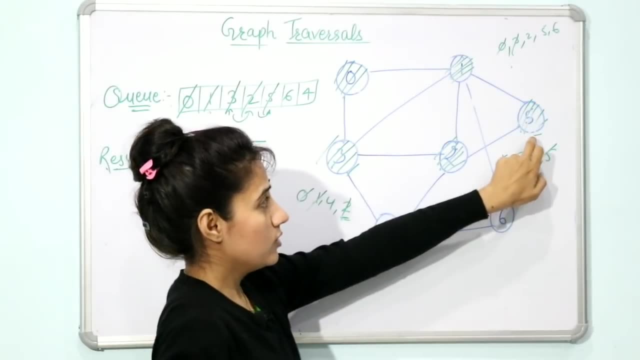 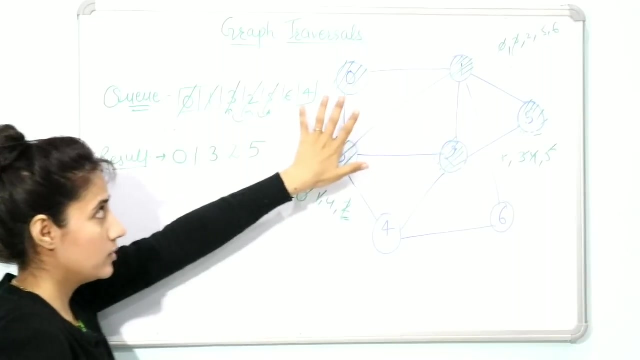 that is 5. 5 is deleted from this Q and 5 would be printed means 5 has been visited. now find out adjacent vertices of 5: 1 we have, or we have 2, but these are already visited. don't know what this is there to be inserted in this Q. okay, 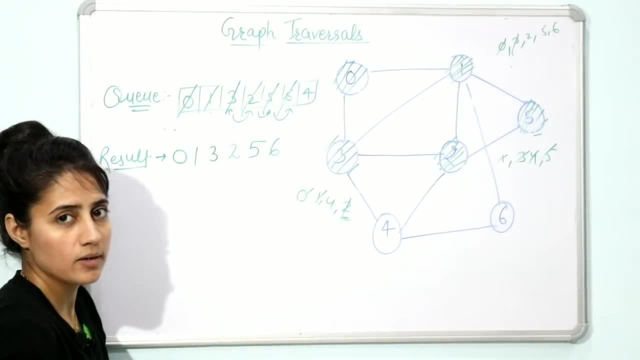 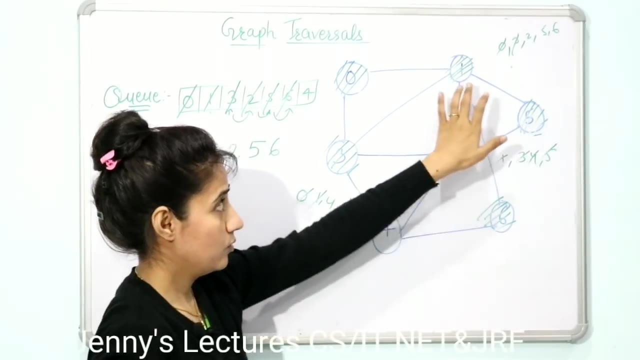 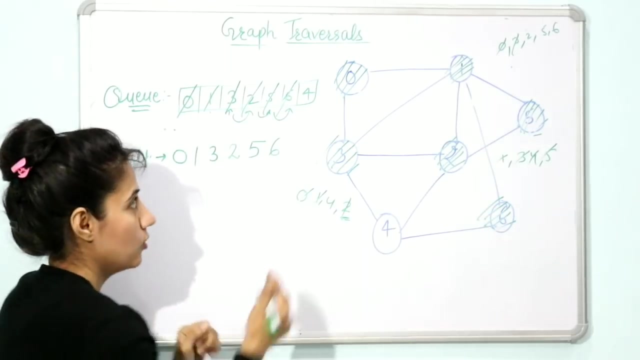 now check the next 6. 6 would be deleted and printed fine. 6 means already visited. adjacent vertices of 6 are 1. we are not supposed to insert this one because this is already visited and one is four. but four is also there, so you will not insert this one. so next you have to delete four and 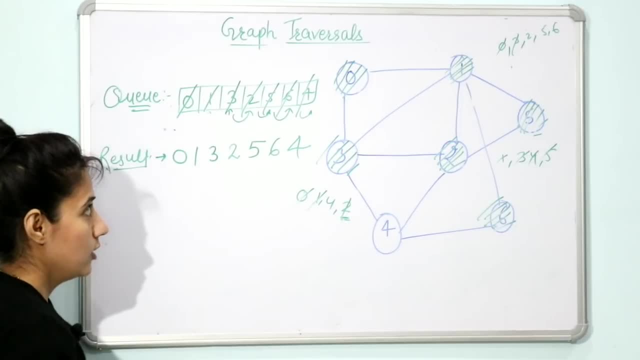 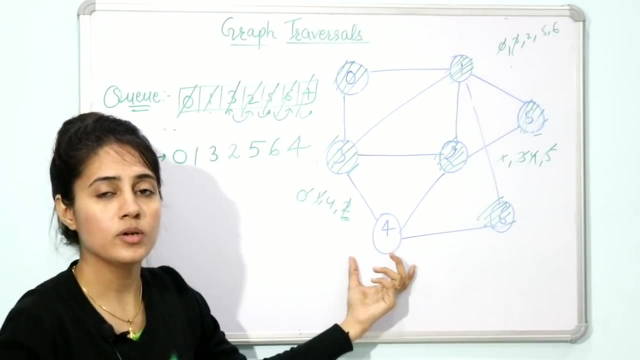 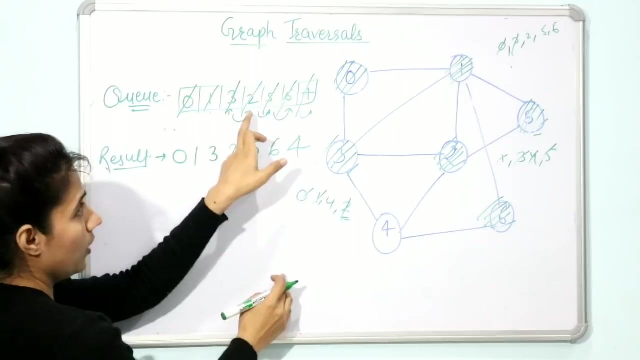 four would be printed fine. so this is the bfs traversal of this graph. see, this is not the only bfs traversal of this graph. there are numerous valid bfs traversals of this graph. how see, suppose you have inserted this two, five, six in this fashion: five, six and. 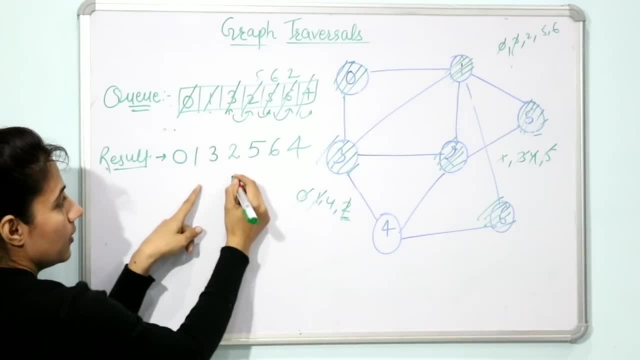 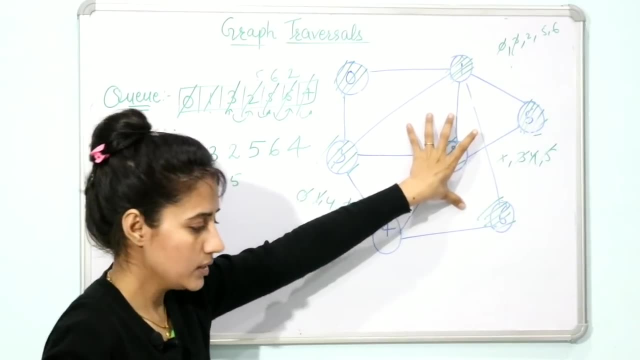 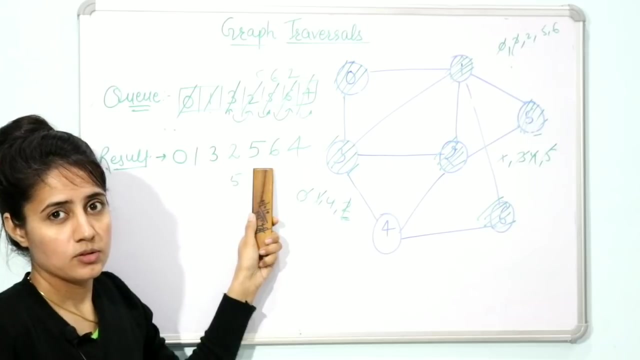 two. so after zero, one, three: what comes here? five comes here. fine, so it depends how you are going to insert these numbers into this cube. so i am not saying that this is the only valid bfs traversal. you can find out numerous valid bfs traversal of this graph, so this: 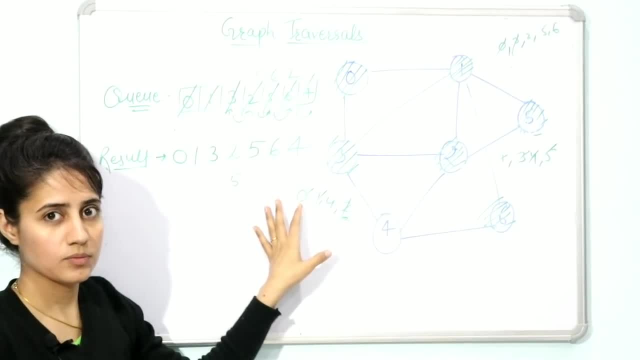 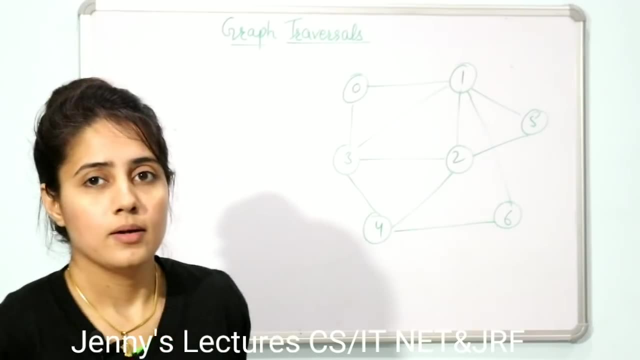 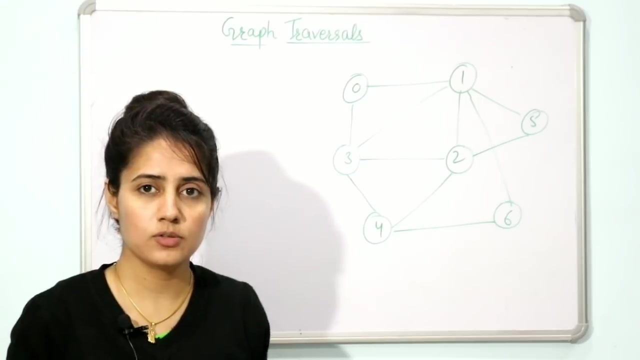 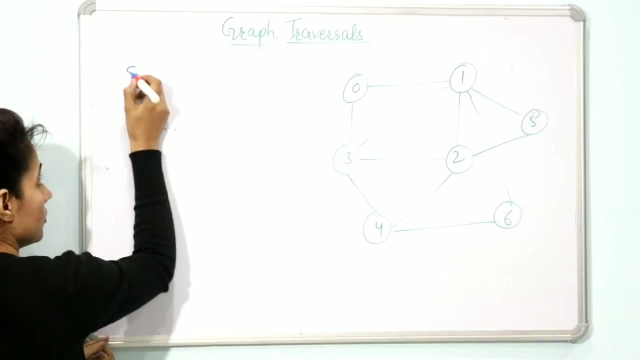 is the only valid bfs traversal of this graph using this method. fine, now we will discuss the dfs traversal of this graph. now we would find out the dfs traversal of this graph. dfs means depth, first search traversal of this graph. okay, in bfs, queue data structure is used and, as in dfs, what data structure will be used. that is stack and it works in leaf. 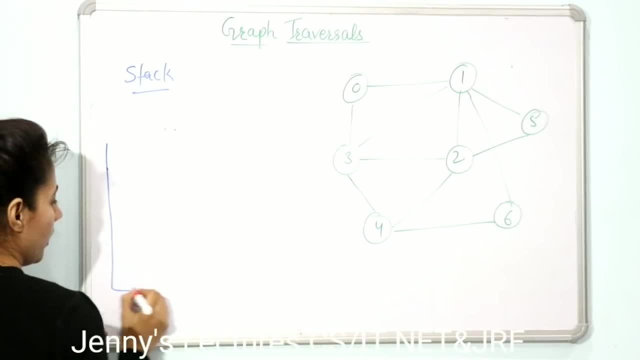 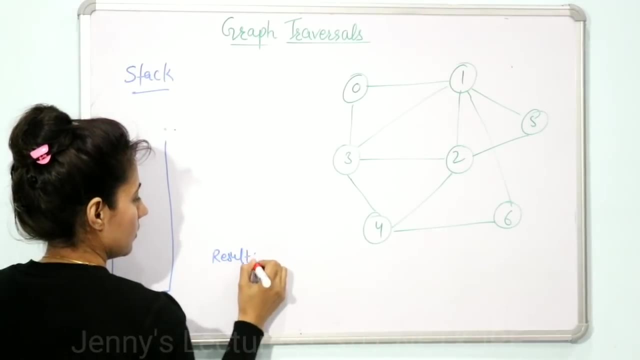 form and it lasts in Gaelic also continuous. most often in bfs the DFS number and the symbol doesn't connect well. as well as in bfs we don't have any string in g, MY P site, and when we took a simple philosophical coke structure and we had two subsr Mcitions, so in my BF we started on. 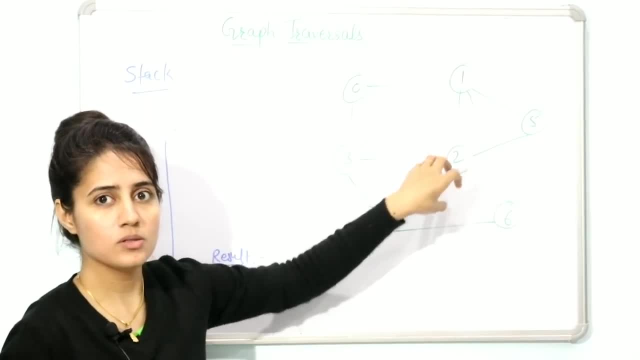 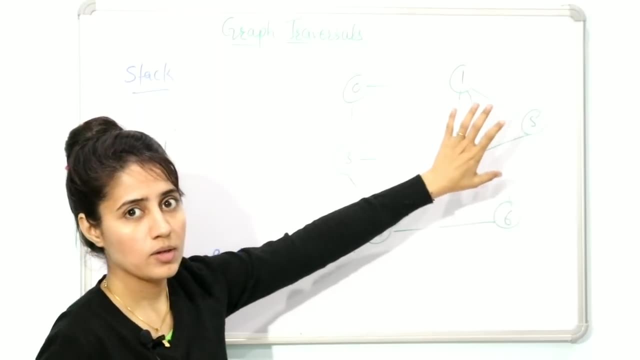 dfs. DFS而且 an Помours BF means that this particular code has a correlation against the standard root, that is the. so it can be taken that the same value does not come out, but the same value reduced some one that I am licking, the same value or different, kinda. 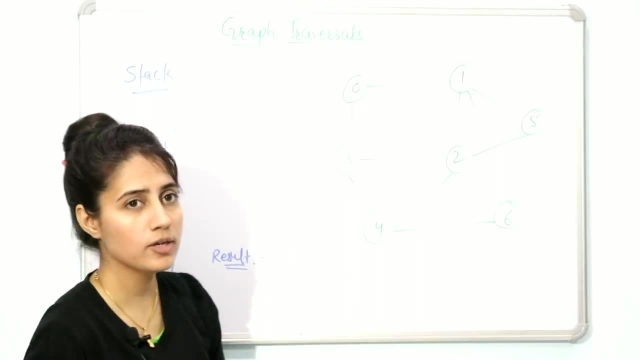 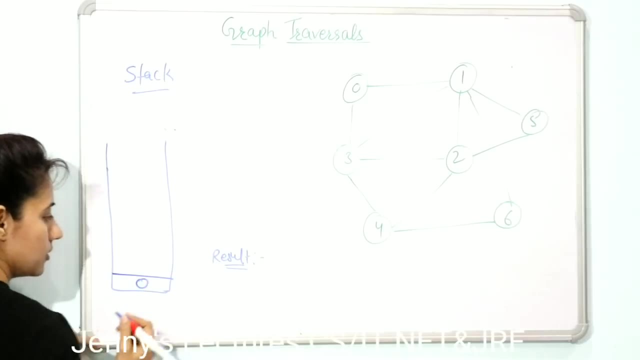 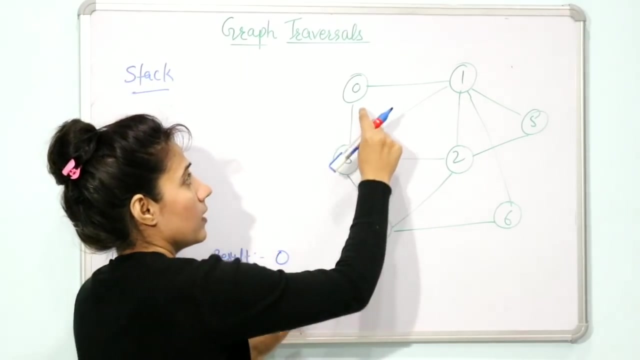 given here, so you can take any node as root node. suppose we are taking 0 as root node. okay, now see, 0 would be inserted in this stack. fine, and 0 would be printed. okay, now check how many adjacent vertices of 0 are there? 1 and. 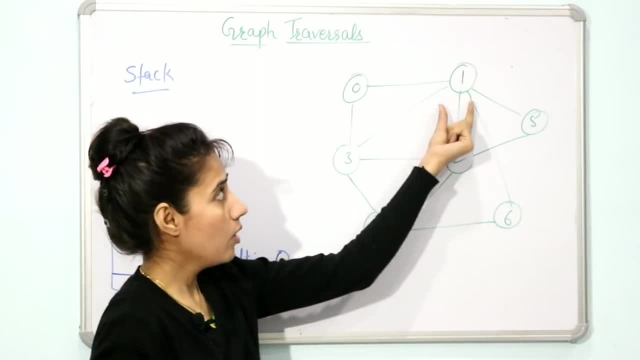 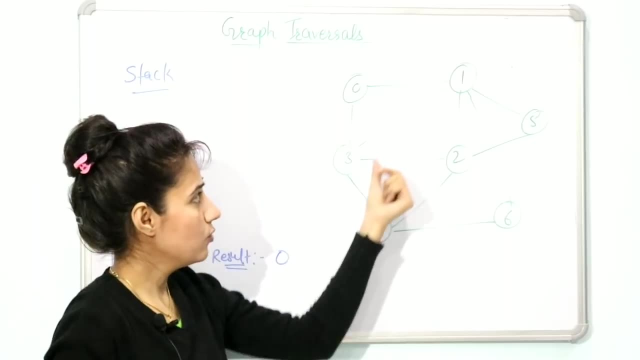 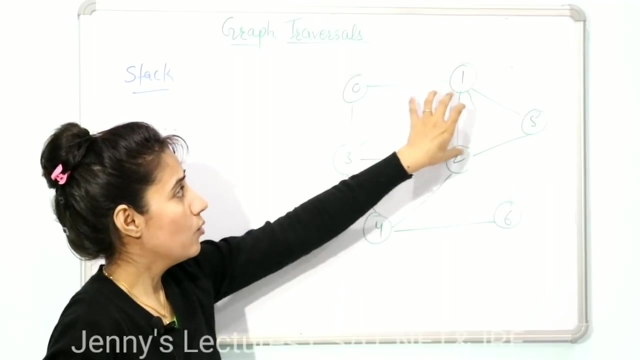 3. so BFS me humne kya kya tha. all the adjacent vertices of that node jo humne q se delete kiya, aur jisko print kiya hai uske saare adjacent vertices ko humne kya kya tha. we have inserted into Q, but BFS me kya hoga? only one, any one of that. 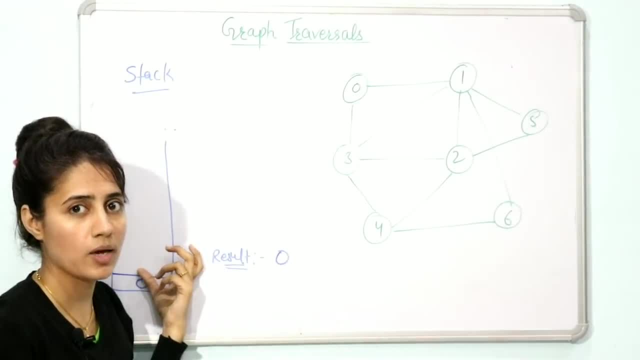 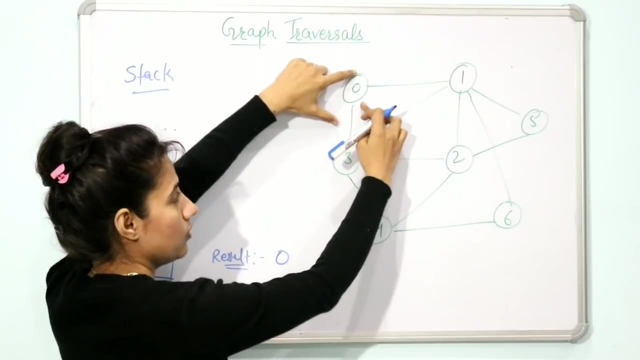 node would be inserted into stack. depth first, search pehle hum depth: me jayenge suppose 0 ko humne ki. after that we have chosen this 3. fine, then we would go through this stack, and then we would go through this stack, and then we would go. 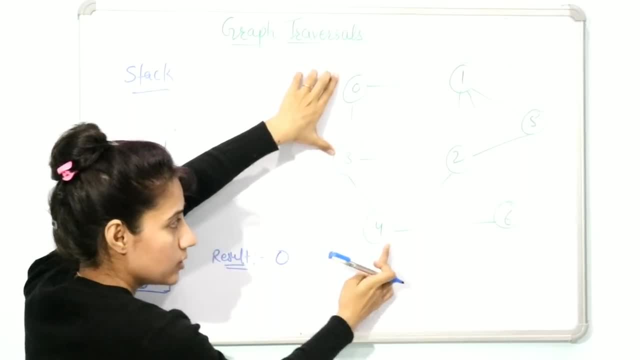 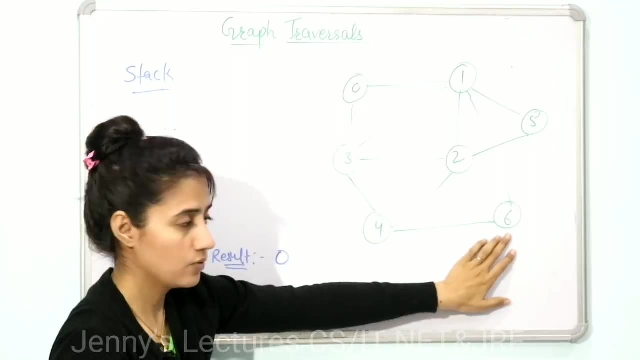 3 to next, iske adjacent me jitne bhi honge, 4 hoga. suppose 6 hua or something like that. at some points we reach. suppose we have reached at 6. fine, and iske aage suppose hum m непas jaane ke liye kuch ni hai. this, this 1 to 6, is not. 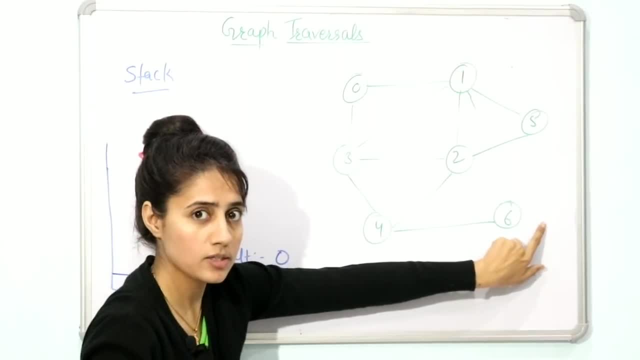 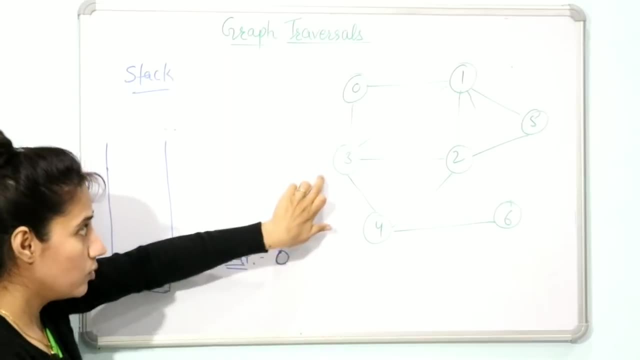 there. let us consider toh 6 ke baad. aap kahin hi ja saktay. after that you will backtrack. you will go to 4 uske baad, 4 ke adjacent me javant ke incase arako kuch ne milta toh then you. then you will backtrack. 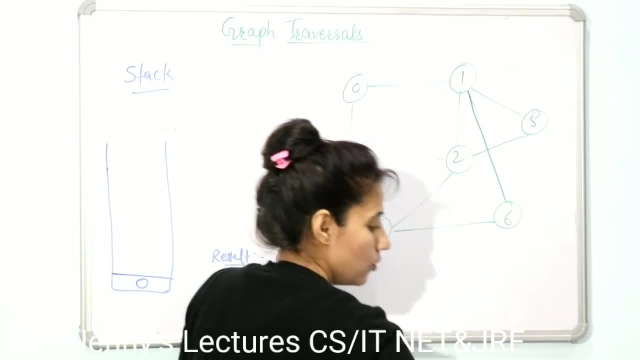 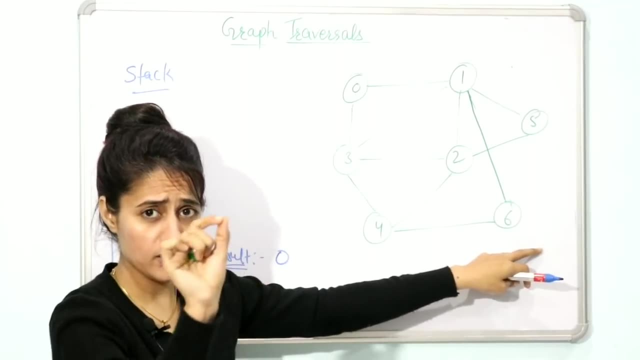 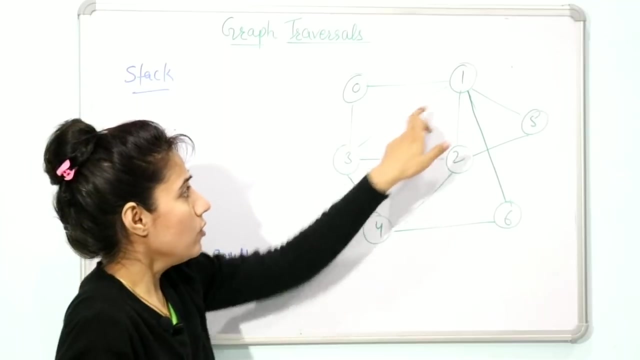 fine, but depths first, search matlab. you will go deeper and deeper until a dead end. dead end means uska, adjacent, unvisited, adjacent, kuch bhi nahi hogay and you have to backtrack. fine, so any one of this vertex zero hai. zero is printed to any one of. 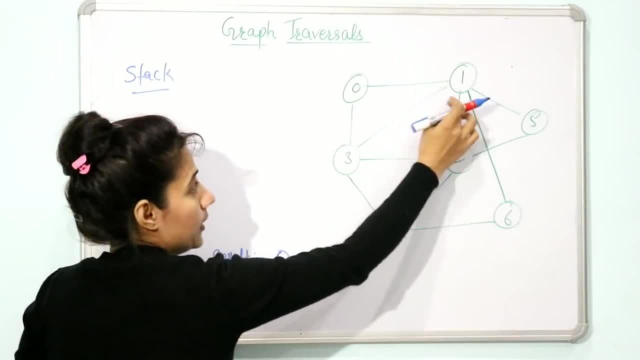 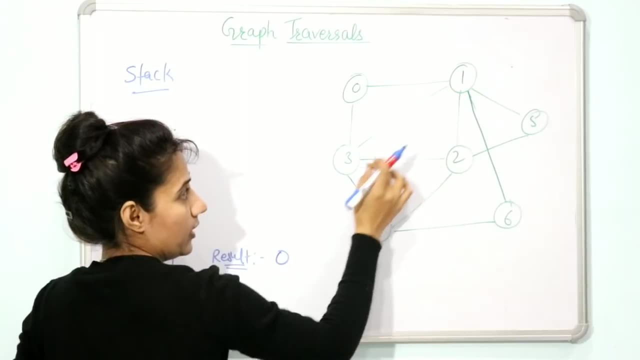 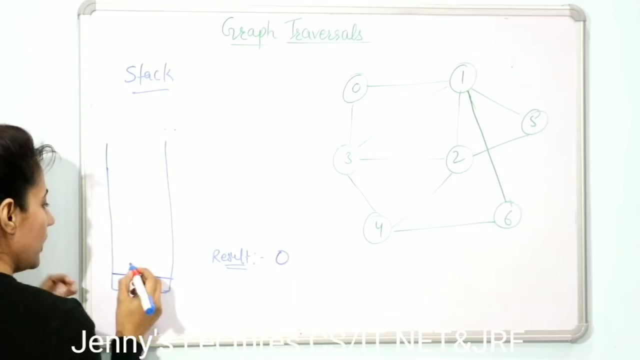 this zero would be taken. any one adjacent vertices of the zero would be taken and pushed into this stack. suppose we have one, we have one and three, two adjacent vertices of zero we have. so you can take either one or you can take three. suppose we are taking one, one would be printed and one would be pushed into the. 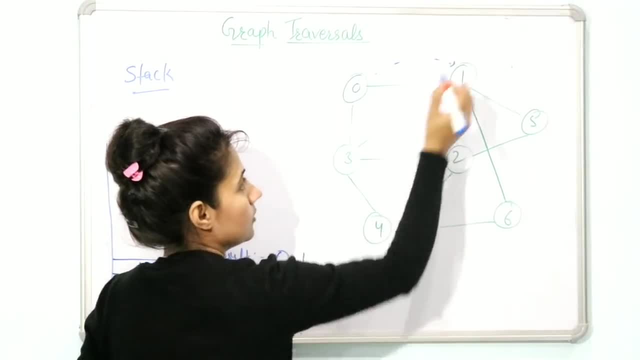 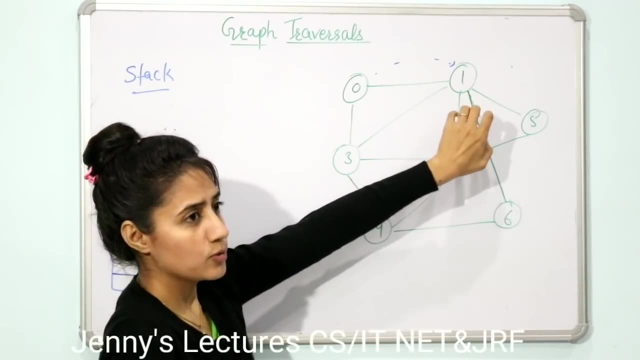 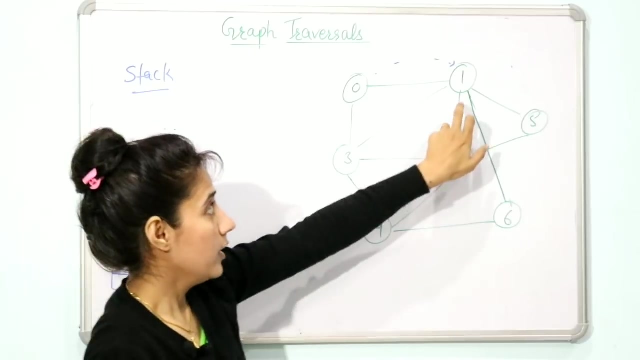 stack zero ke baad hum kahaan pe gayi hai this one. after that you would explore this one. explore nahi, explore means explore. karnah hota hai, ki ap sare vertices ko aap explore karoge. wo explore hum kya kartayen? bfs, me kartayen now one ka you would take any vertex. 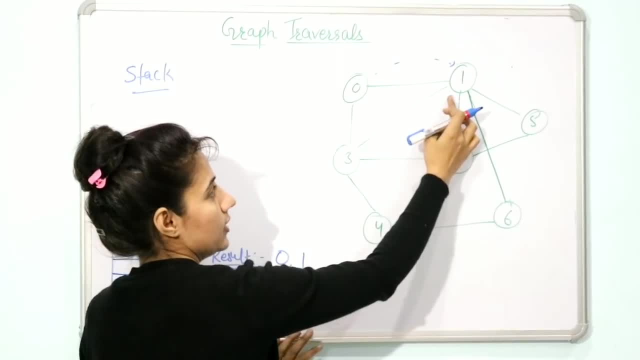 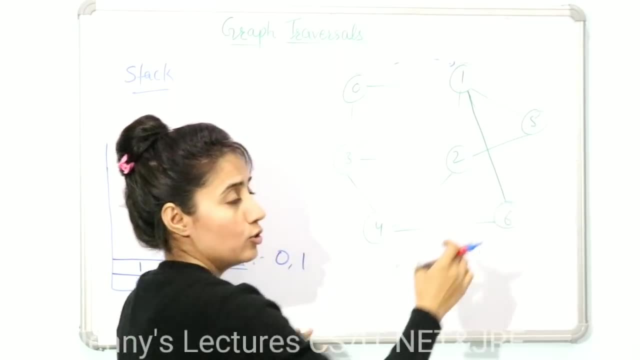 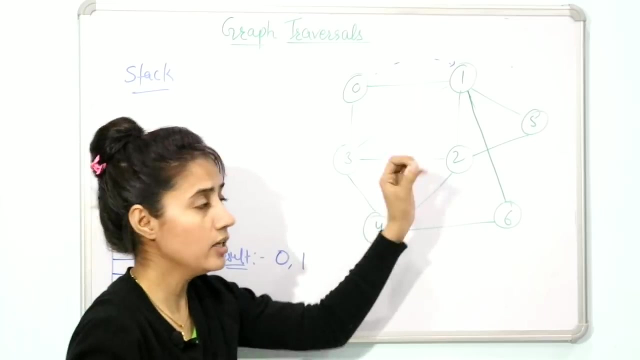 unvisited vertex kutne adjacent vertex one ke adjacent vertex. vertex kaun kaunse humne paas three, two, six and five. fine, so you can take any one of these four bfs ki tarah chaaro aapko insert nahi karna hai. you take any one of these four. 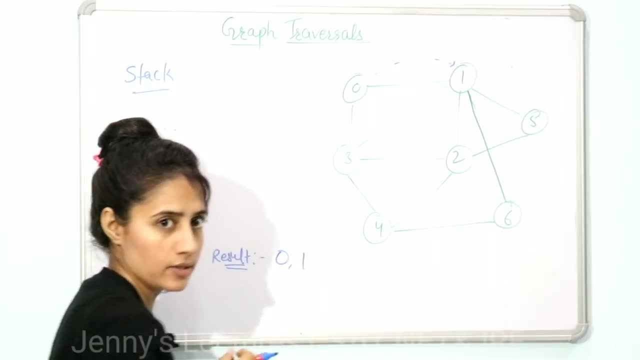 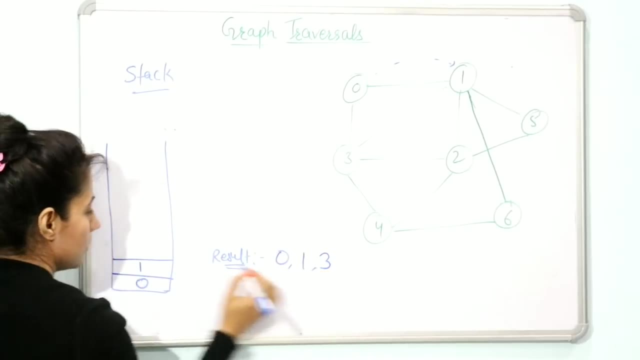 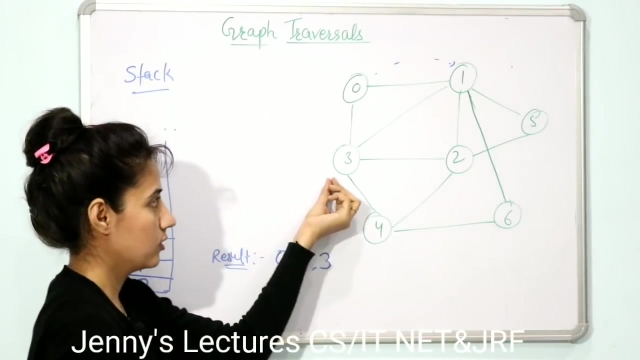 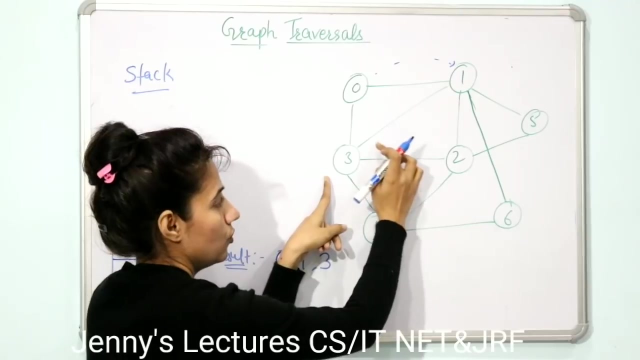 three, two, 5, 4, 6, suppose we have taken this 3. fine, 3 we have taken and 3 you have inserted in the push, in the stack. you have pushed it. fine, so you are now at this 3. now find out adjacent vertices of this 3, this 4, this 2, this 1 and 0, but obviously 0 and 1 are already visited. 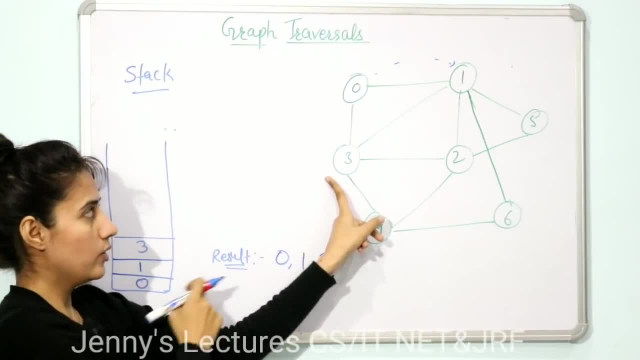 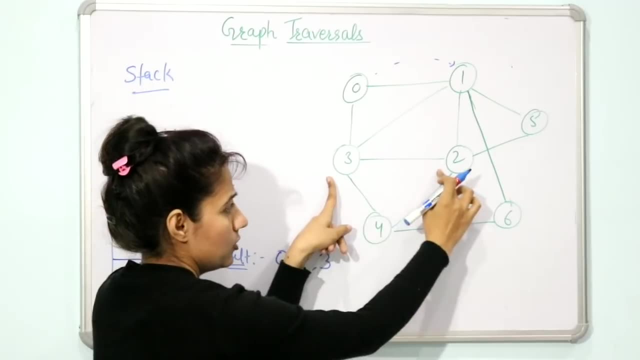 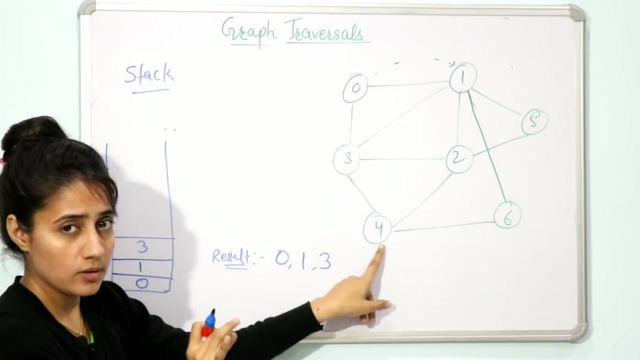 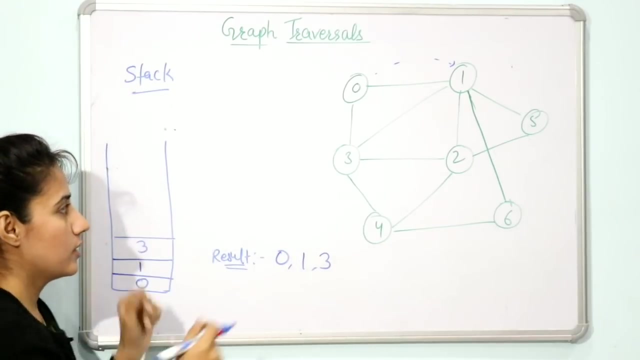 fine, 0 and 1. see in result. see 0 and 1 already visited. so you have to find out: unvisited vertex, unvisited vertex which one. we have, 2 and this 4. so you would take any one of this, these adjacent unvisited vertices, and you would push that vertex into this stack. 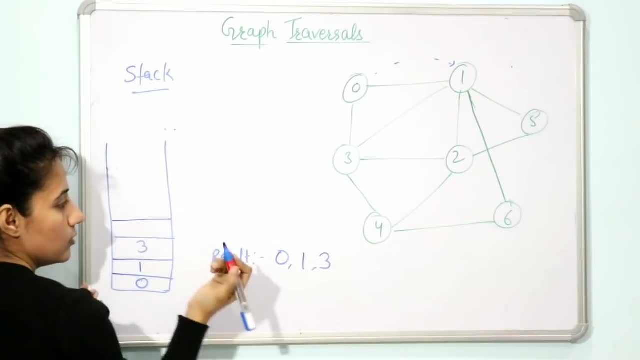 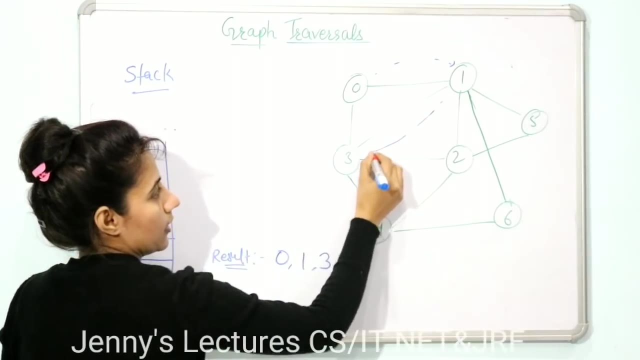 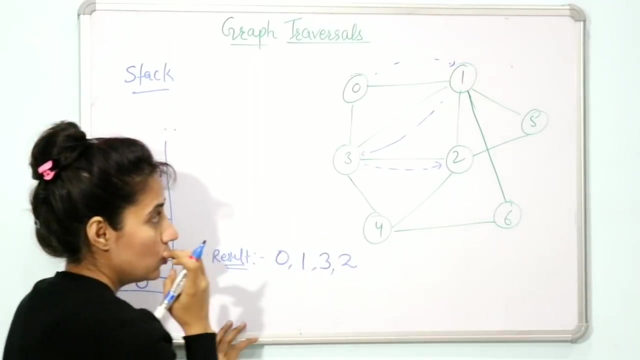 you can take 2 or 4. suppose you have taken 2, 2 you printed 2 and you pushed 2 into this stack after 3. where have you gone? 2? fine, now you are at this 2. now find out adjacent vertices of this 2. fine, which are its adjacent vertices? 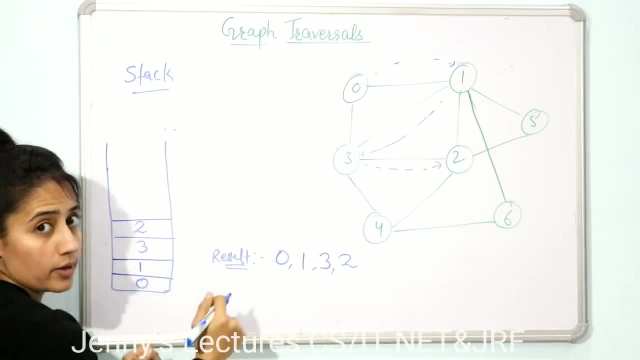 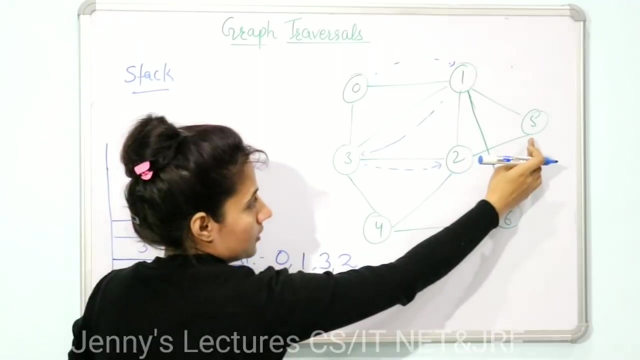 1, but you cannot push 1 at this one because 1 is already visited. you cannot push 3. 3 is already visited. now you have remaining adjacent vertices 5. you can push 5 into this 2 and 1. is this 4 adjacent vertex? fine, this 5 and 4. so you can take either 5 or either 4, any 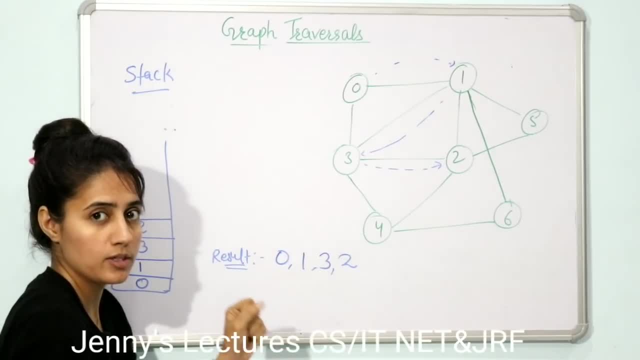 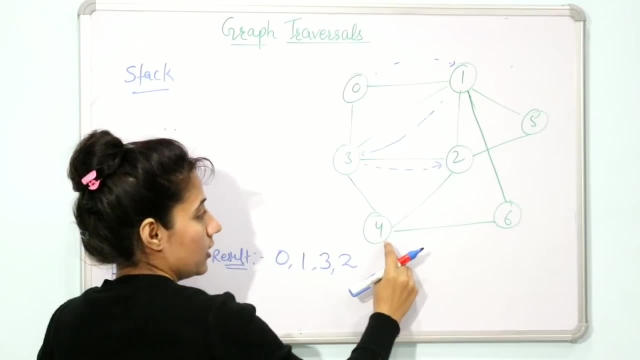 1. ok, you don't have to take all of them. I am focusing on this again and again: any 1 you have to choose. that is unvisited vertex, and it should also have adjacent vertices, so you can take either 4 or 5. suppose we have taken 4, we have pushed 4, and where have you printed? 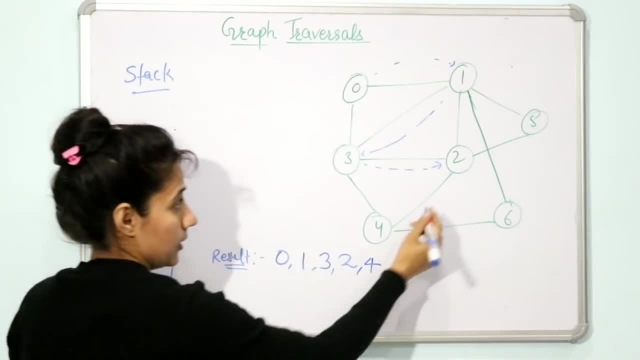 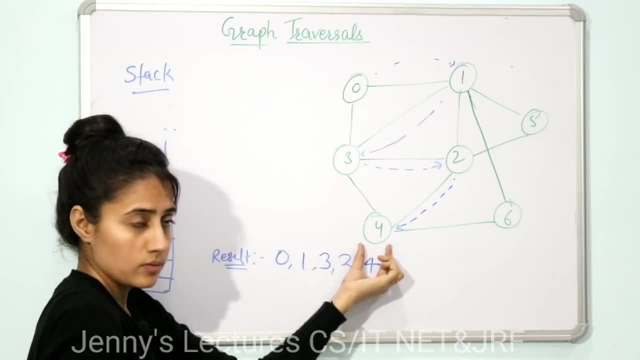 4 on this stack, so you can take either 4 or 5. suppose you have taken 4, we have pushed 4, and where have you printed 6 and 5? so you can take either 5 or 5, so 6 or 7 each then. 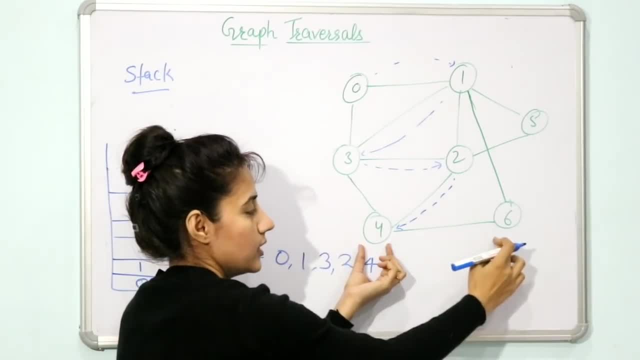 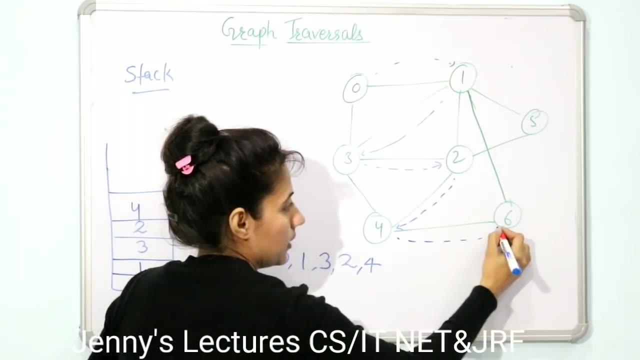 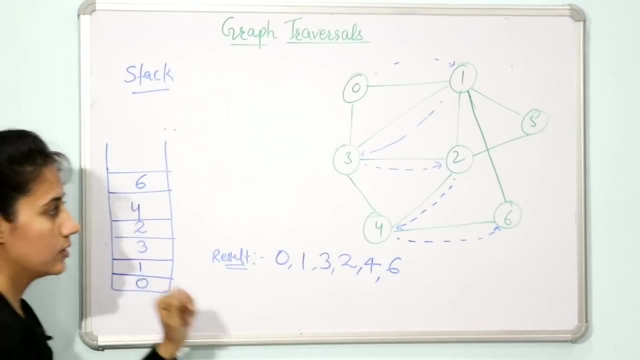 where are you printed 2 and where have you looked at? you can take both of these and put this back above the vertical axis. 2 and 3. fine, so now the objective is to make of Arra is that it should not be placed in the good one. V. and then what is the objective of 209? ok, we go on with now. at this point, see hasta. this line is連 words. keep in mind that 6- there was a Mercer in this line- 4, this line is 1 and the opposite ring goes to the 2, first number. 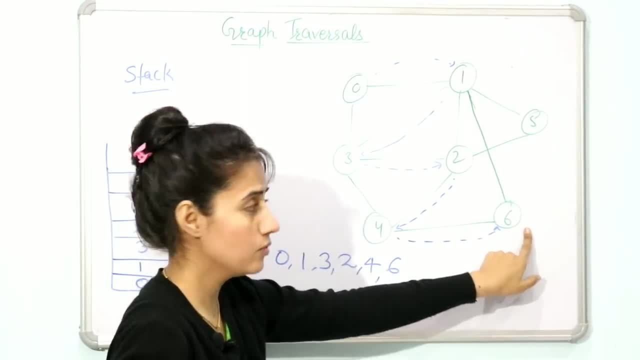 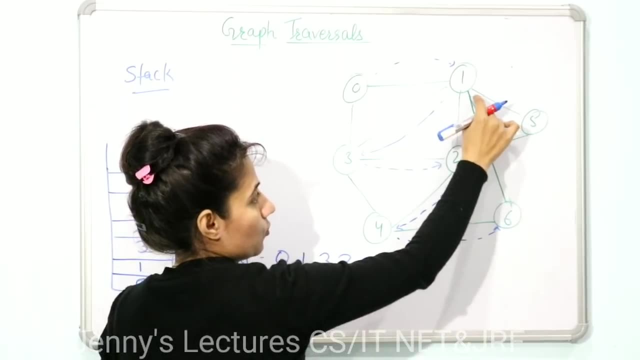 Is there any unvisited adjacent vertices of 6?? Its adjacent vertices are 4, but 4 is already visited. Adjacent vertices of 6, 1 is 1.. 1 is already visited And we have only 1 and 4.. 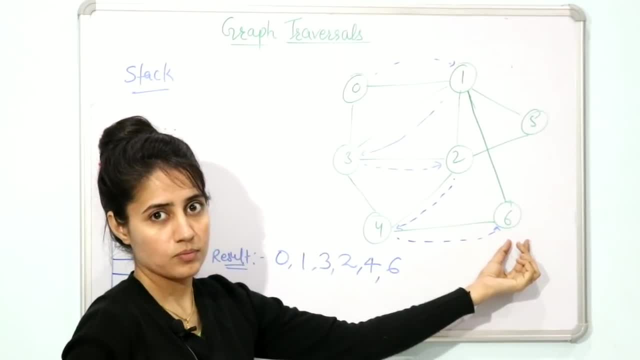 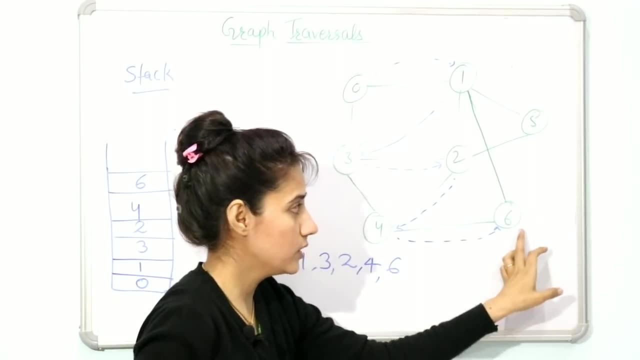 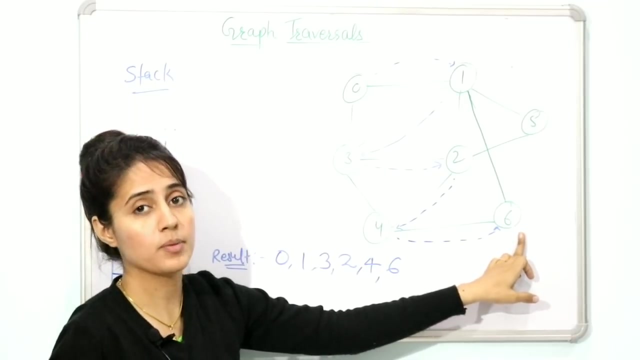 So no unvisited adjacent vertices, is there? Fine, What will happen here now? You cannot move further from the 6. You cannot go after 6 in deep Because you do not have any unvisited adjacent vertices of 6.. Where you can go. 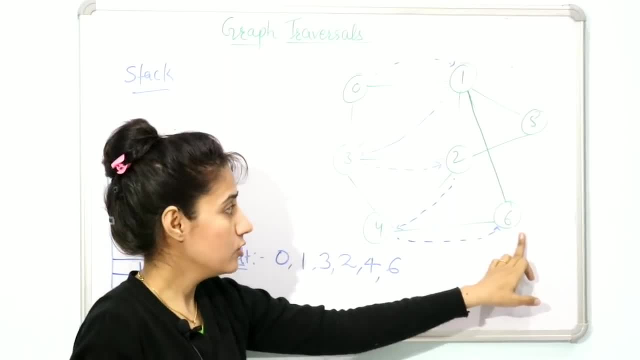 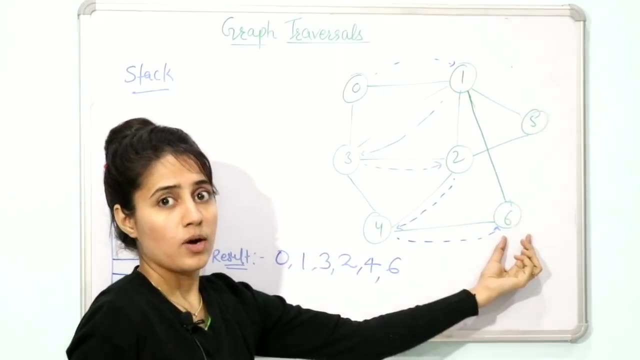 So what will happen here? Backtracking Now. how will backtracking happen? How will we know where to go in backtracking From this step If such a situation comes? what happens there? That step is there. The topmost element is deleted. 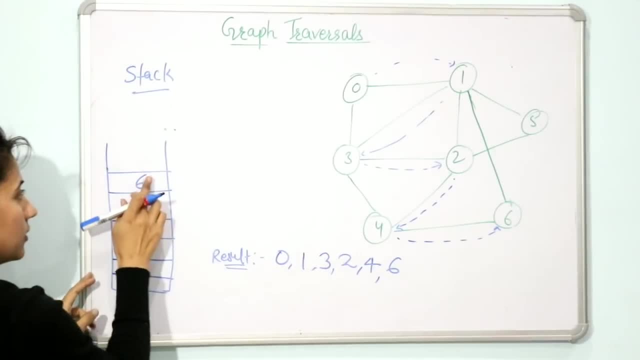 Popped out. Or you can say: popped out, Then 6 would be popped out. 6 is pooped out, 6 is pooped out. Fine, Now See, the next top element is 4.. Now, this will tell us that from 6 you would go to which element. 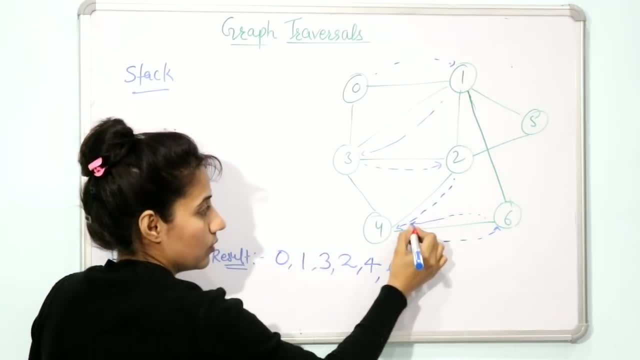 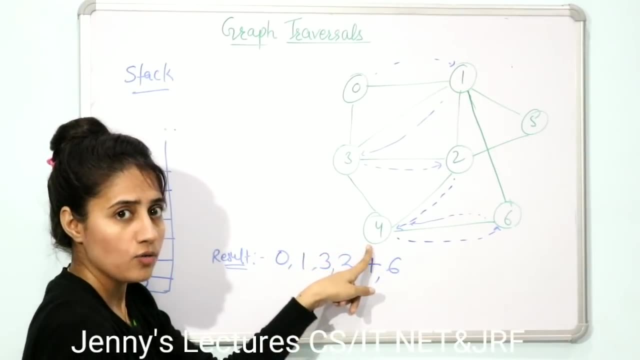 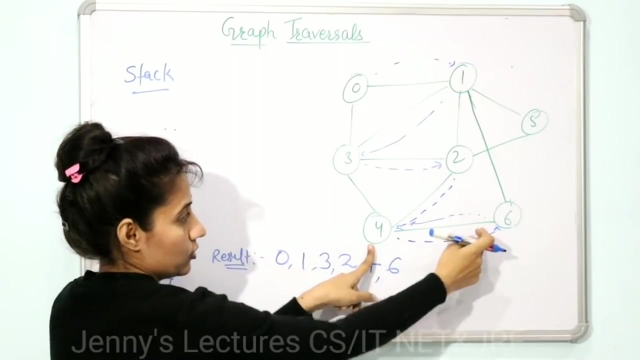 This 4 element, Then backtrack to 4.. Fine, Now check This. 4. has any unvisited adjacent vertex still? Is there any 4?, 3,, 2,, 6, all are visited. No vertex is there Then 4.. 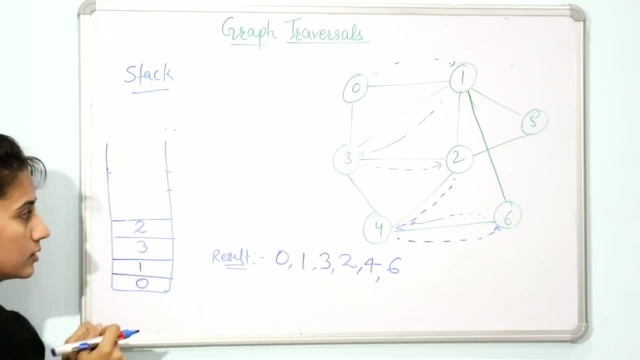 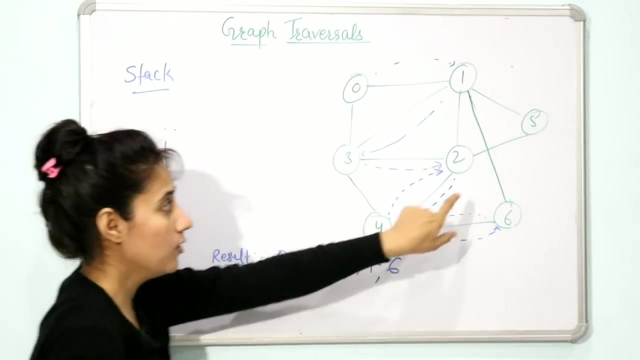 5 would be popped out from the stack. Next element is 2.. Now we would go to 2.. Backtrack to 2.. Now find out, Is there any adjacent vertices of 2 that is still unvisited? Yes, we have. 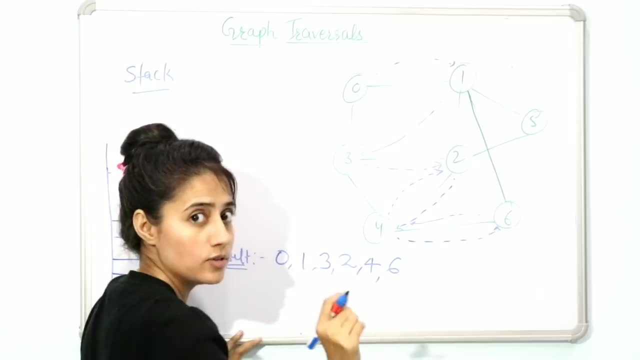 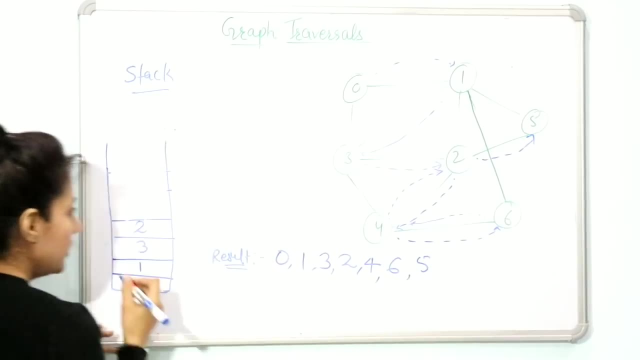 What is that? This 5.. This 5 is still unvisited And it is adjacent of this 2. So we would go to this 5. 5 would be printed And 5 would be unvisited, And 5 would be pushed into the stack. 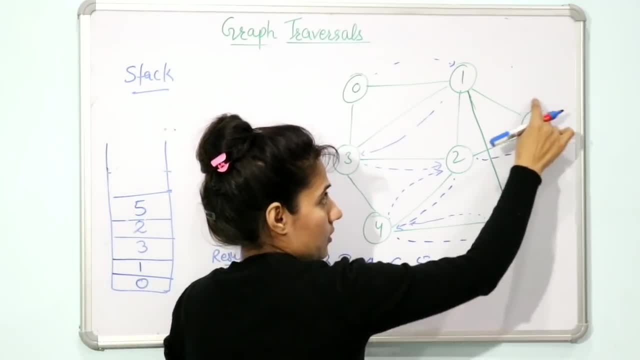 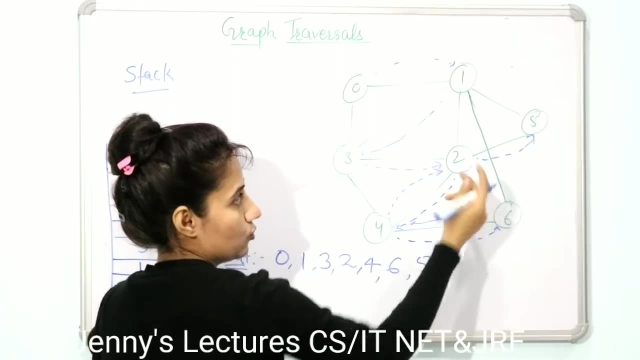 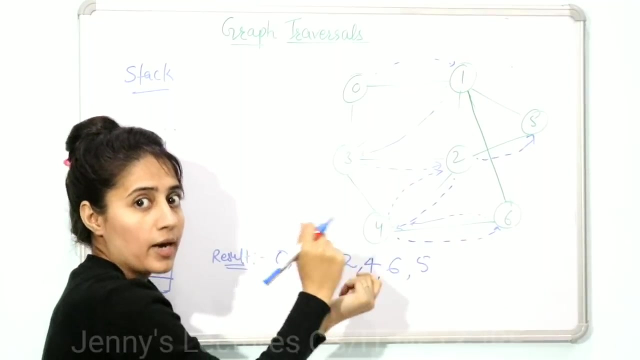 Fine, Now check 5.. Is there any adjacent vertices of 5 which is still unvisited? No 1 already visited. 2 already visited. What the next step is? We cannot go further from 5.. So you have to backtrack. 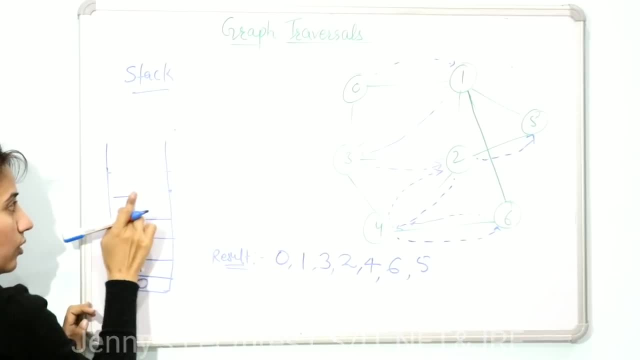 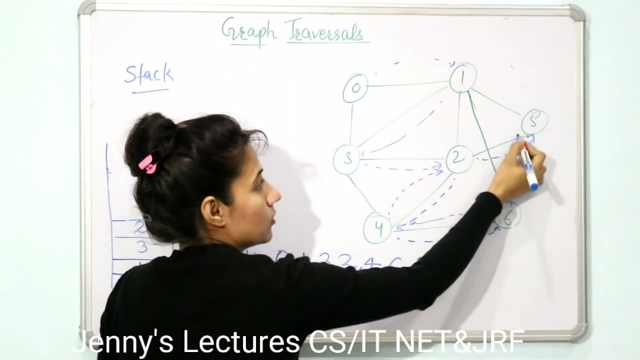 Where do you have to backtrack? First step is 5 would be popped out from the stack. Ok, The top element would be popped out. Now check the next top element. That is 2.. Then where will the backtrack come from 5?? 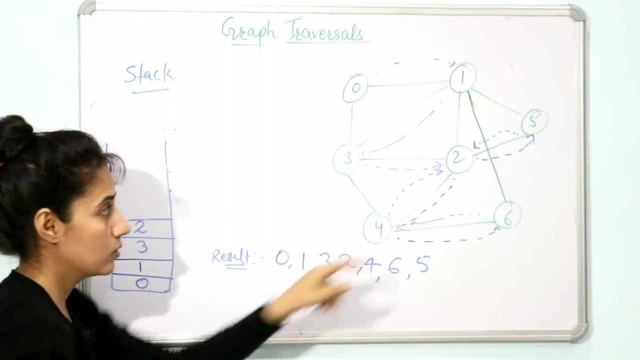 To the 2.. Now check: Is there any unvisited vertex of 2 that is adjacent of 2 and still unvisited? No one is there. Ok, Then pop out this 2. Now. next is 3.. So where will the backtrack come from? 2?? 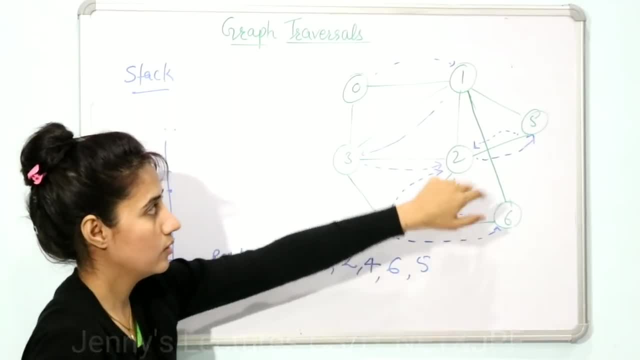 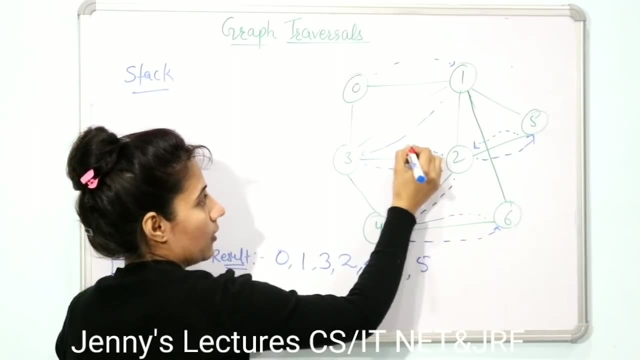 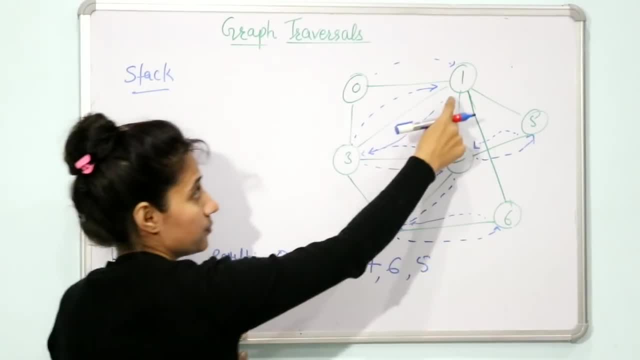 2. 1. 1. All are visit, Then pop out this 3 from the stack And next is next. top of the stack is 1.. So from 3 we would go to 1.. Whatever is the top of this stack, we go there. 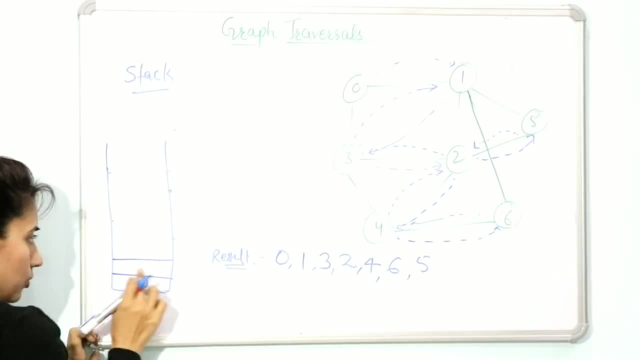 See, is there any unvisited adjacent vertex of 1?? That is, you can push into the stack. No, All vertices are visited. That is which is adjacent. So pop out this One from the stack and find out the top. 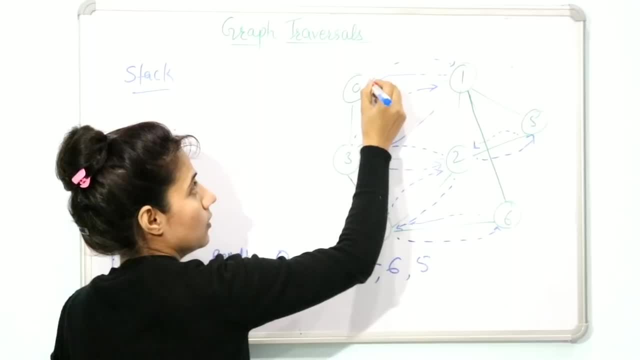 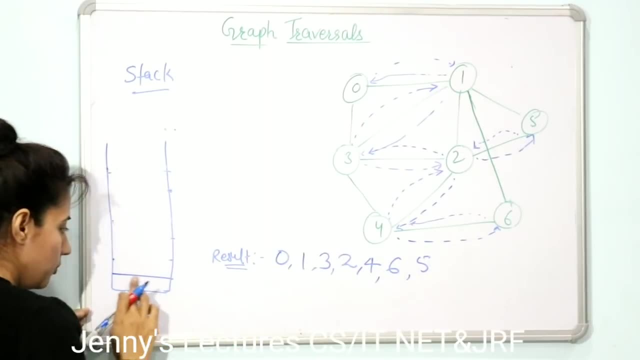 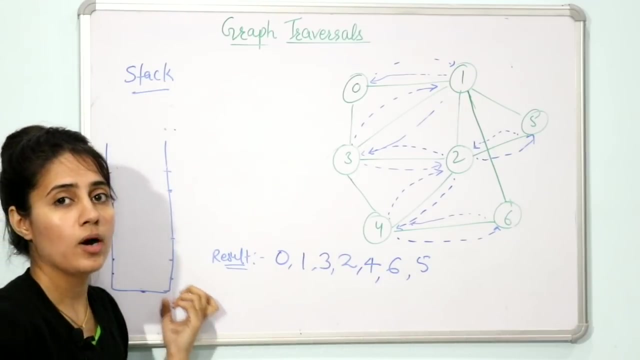 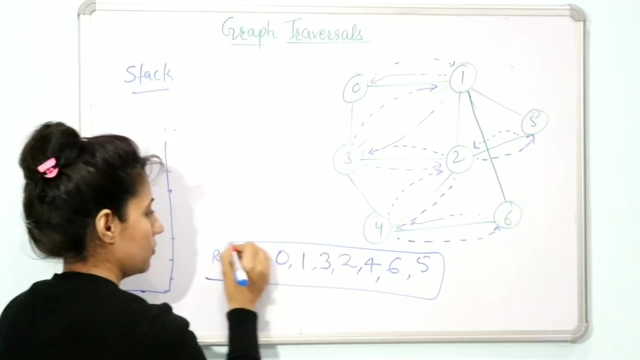 is zero. now from one we would go to zero. find out zero ka koi hai. adjacent vertices: that is still unvisited. no, then pop out this zero from the stack. now see, stack is empty. so this is the indication where you have to stop this dfs algorithm. fine, and this is the dfs traversal of our 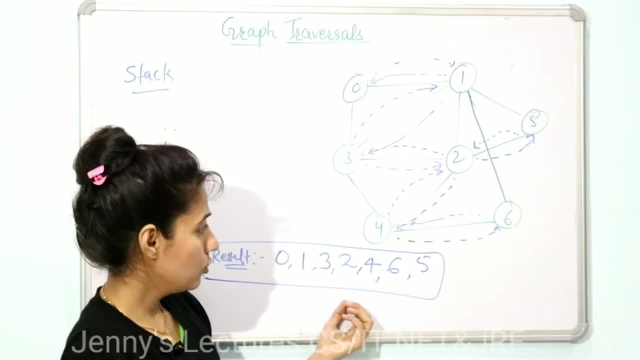 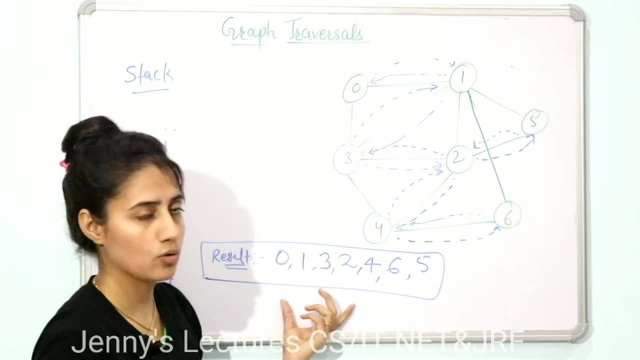 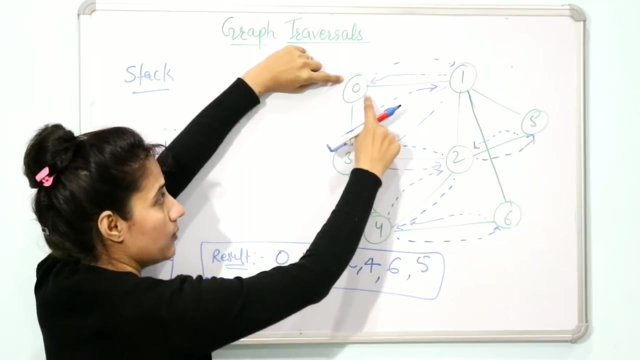 graph. now, in this case also, this is the only you know. this is not the only dfs traversal. there are numerous valid dfs traversal of this graph. how you can find out, see, suppose you are starting from zero. hum yaha se zero se start kar ke hum kaha gayi the pehle to one, but from zero. 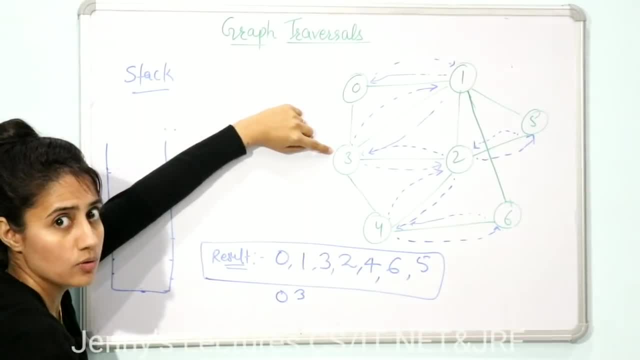 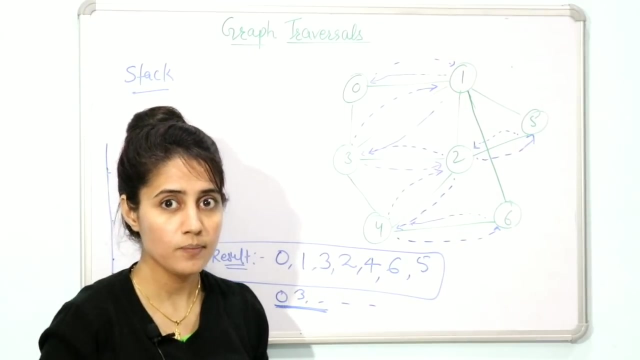 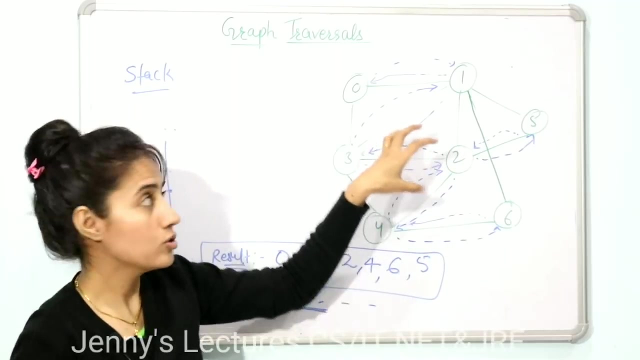 you can go to this vertex three also take a uske baad a visit karoge to this would be another dfs traversal, fine, so aise bahut saare isme dfs traversals hapke ho sakte hai to bfs. maine aapko bata diye hai bfs me kya hoga. try to explore all the nodes as close as possible.